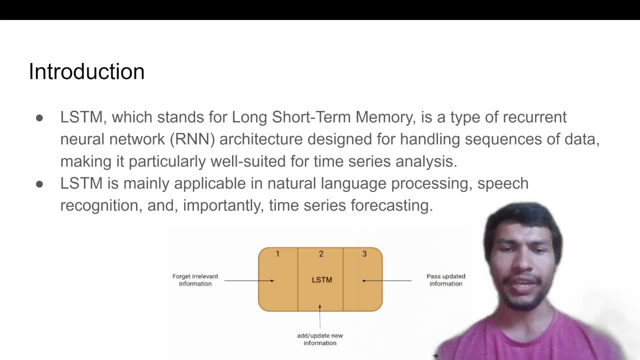 and then, in the second step, it try to add or update the new information, which of course, achieved by training the model, and then it will pass the updated information to the model and then it will simply loop it and then simply run it for the several time to get the best accuracy. so yeah, so that's how it works. 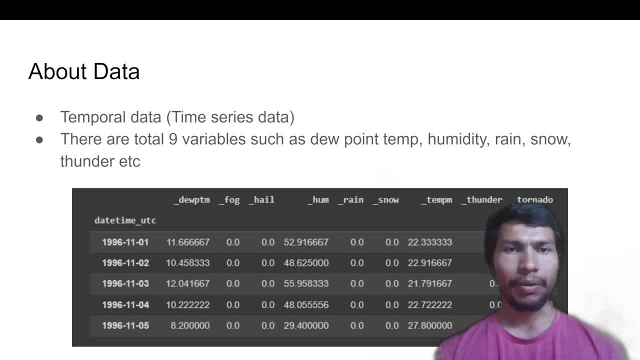 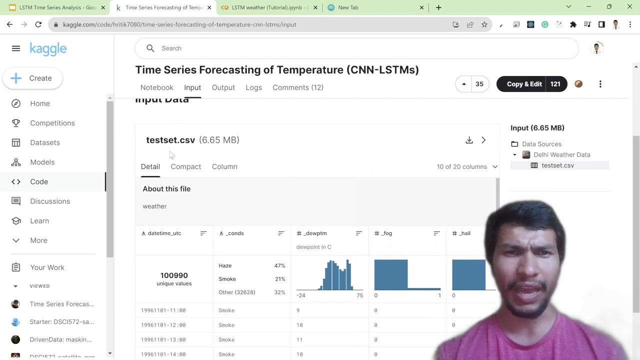 so, talking about my data set, my data is the temporal data. of course, temporal means the time series data and there are total nine, nine variables that I'm going to use, which are like dew point, temperature, humidity, rain, snow and thunder, etc. so the data I got from the Kaggle, so here they have, the test set. 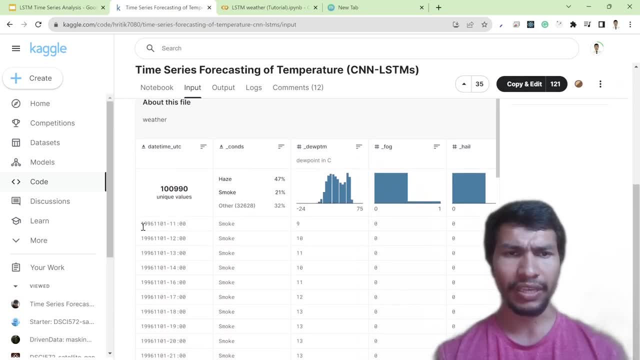 dot CSV file and of course you can see it. it start from 1996 11, which is November 1, to I think it's 2017 or something, and then they have, like hourly data set. so in my model I'm going to, I'm trying to. 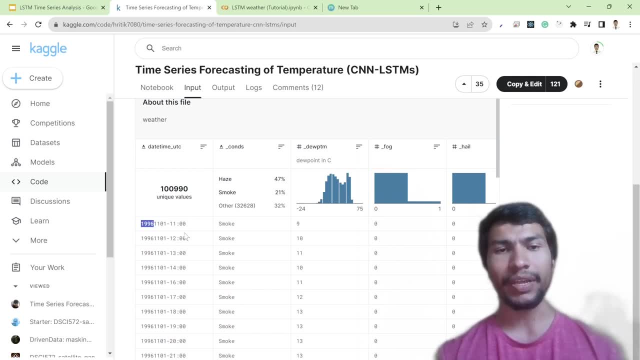 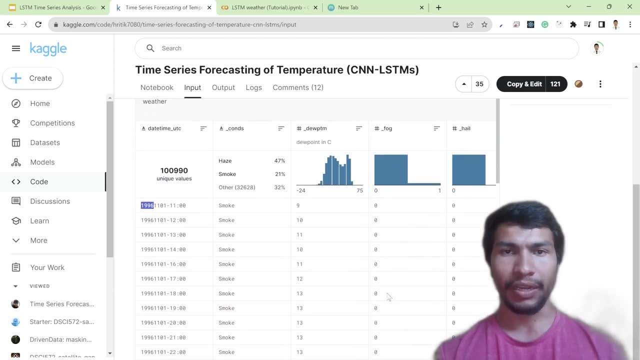 like compress it to the daily data set by averaging the daytime temperature and then try to predict that day average temperature. and here you can see they have like different data set and then they have like the average temperature, and then they have like the average temperature and then they have like the. 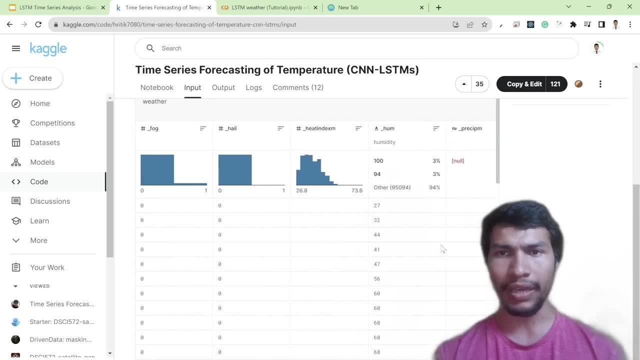 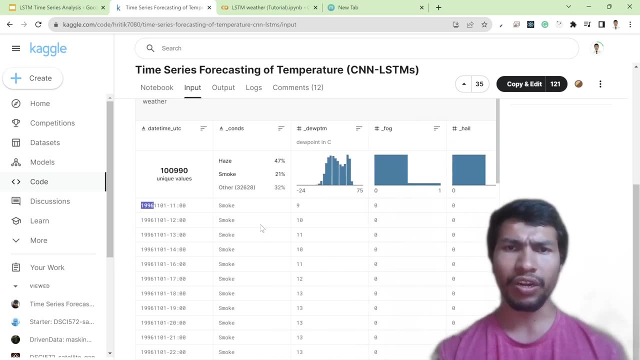 different variables like dew, PTM, fog, hail and heat index. humidity, precipitation- different variables like dew, PTM, fog hail and heat index. humidity, precipitation, pressure, rain. of course we don't need all the variables, so of course you can like you can try with all the variables and then you can try with only two or 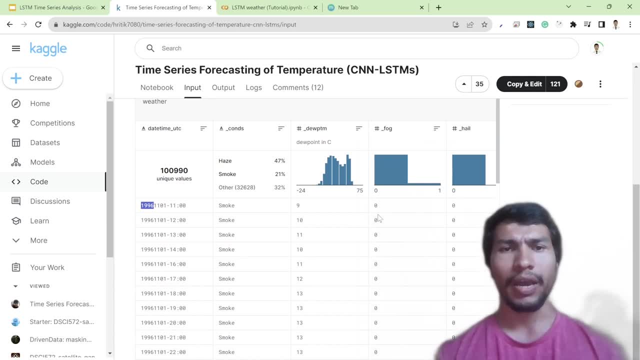 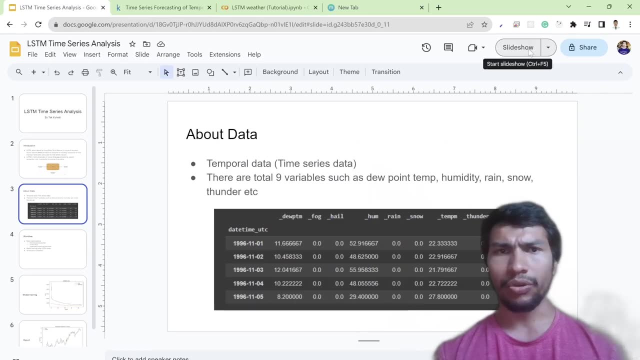 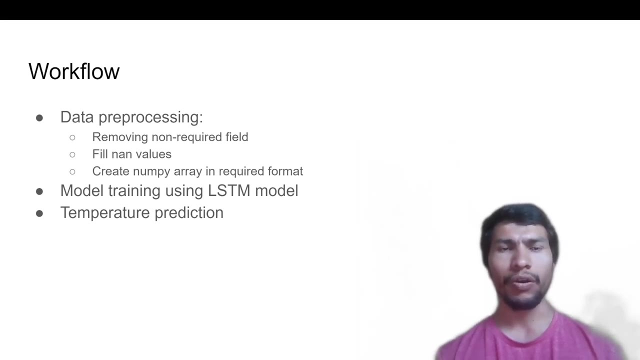 three variables, but for this particular video I'm going to use only, I think, nine variables. so, yeah, let's go to the presentation mode, and okay. so my workflow here is to: first I'll do the data pre-processing, so that means I'll remove the non required field, and then also, there are few like. 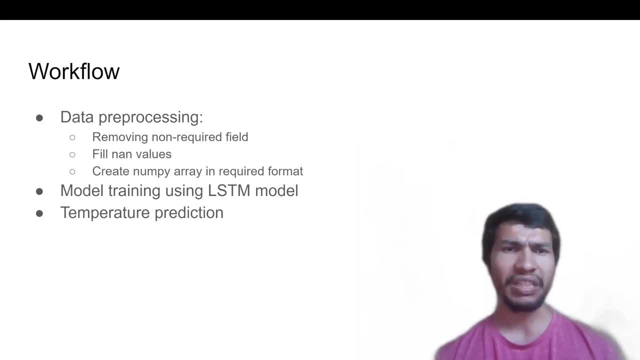 non values. so I'll try to like fill them based on the upper must value, uppermost, like the temperature, and then I'll also create the numpy array in the required format, I mean the required shape, and after that I'll train the model using LSTM model and then predict the temperature and then 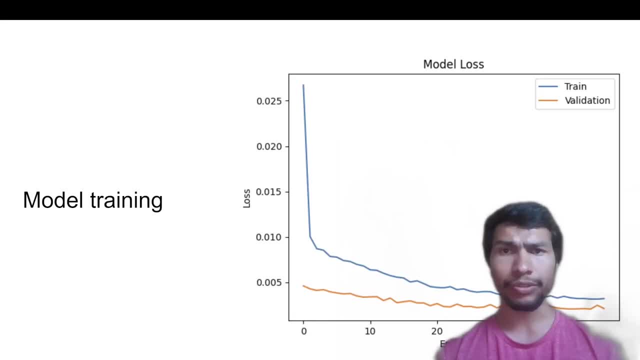 I'll show you the graph in a minute, okay, so I since I already did it. so my loss function, my like history look like this. so in this graph you can clearly see that my model is like improving slightly, my loss is like decreasing. so I'll train and show you after this presentation, and this is the result. so 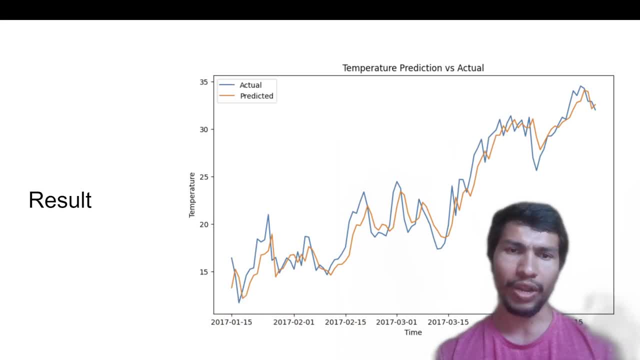 the actual temperature is represented by blue line and then the predicted is in the orange line, so it looks like it has it did pretty good, good job during the prediction, and yeah, of course, I'll show you, so let's let's go to the coding section now. 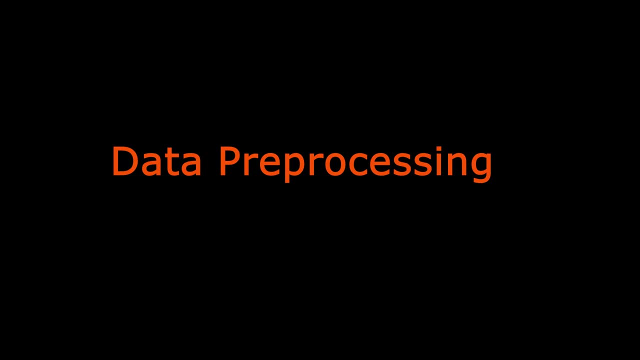 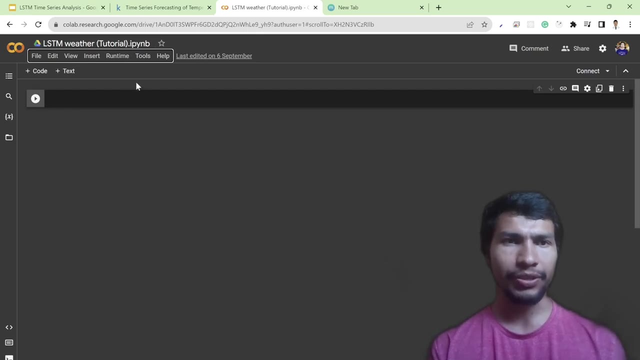 you all right. so for now, I created the like Google collab with LSTM weather tutorial. and here is always: I need to like import the main packages, so I'll import: numpy is NP and then pandas is PD, so that's what I need of in order to pre-process. 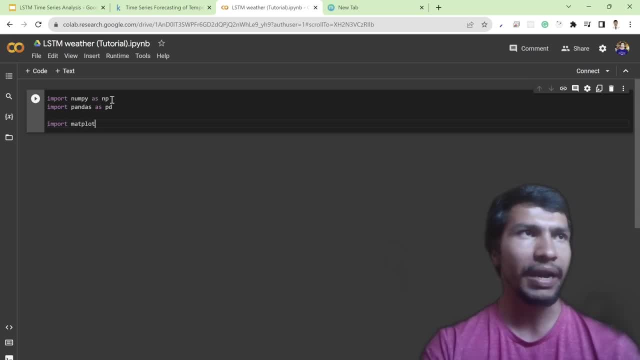 my data set, and I'll show you how to do that in a minute. so let's go to the doc in order to easily incorporate this program and what I will have worked well in just the program다고. so let's go to the note stack and then I've. 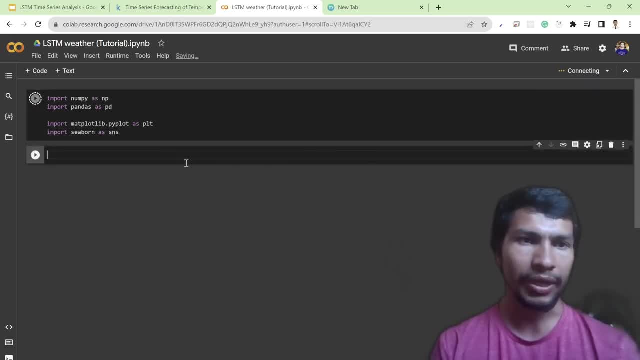 未 was cunhaed needed all know. I can go to the workflow section. I dead. I'll click on HTML orCon weave. what we do here is we're gonna need to type all the things like朋友- I mean, this gets asked every often- like click the. 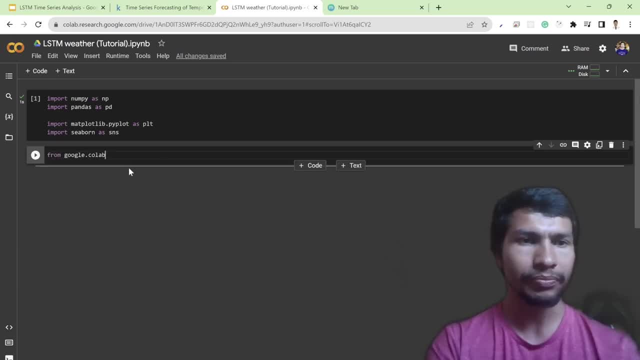 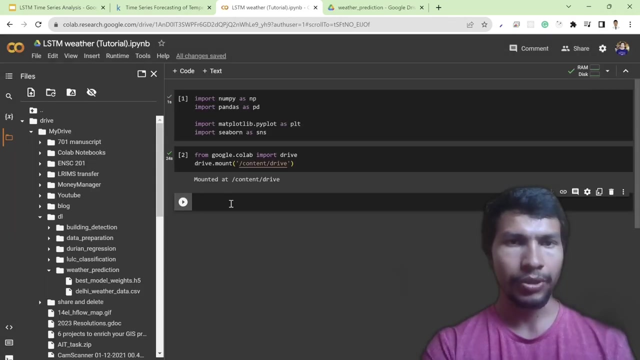 other function that click on viewers in theциelsak like Google collapse, so I'll write from googleco lab import drive and then I connect my drive, dot mount and then slash drive. okay, if you connect the drive properly, then you can see your my drive drive folder over here in the 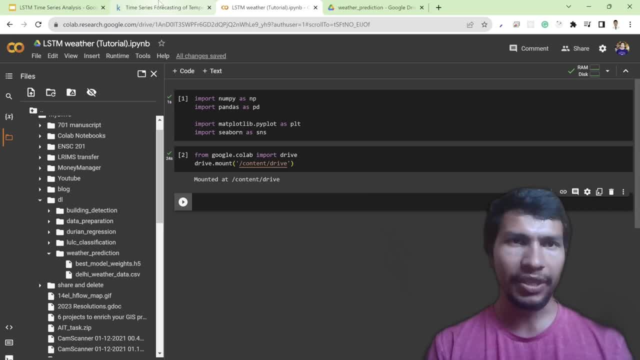 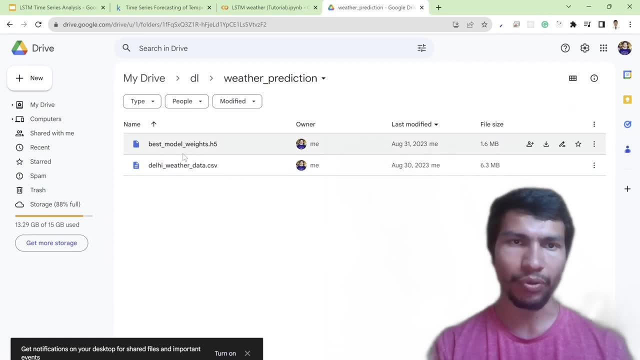 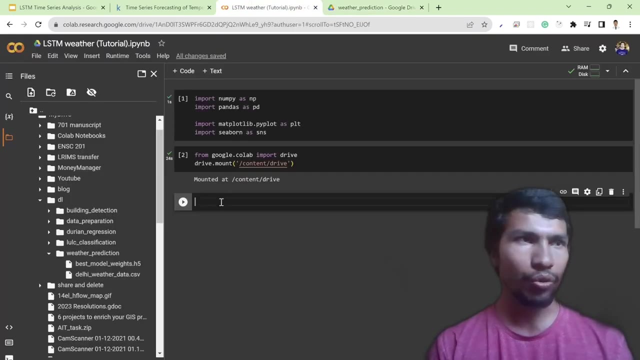 folder menu, file menu, and make sure you download this data set from here and then upload it somewhere in your drive. so I renamed: the file name is the live weather data dot. CSV, and so after that you can see that the file name is dillyweatherdatacsv, and so after that. 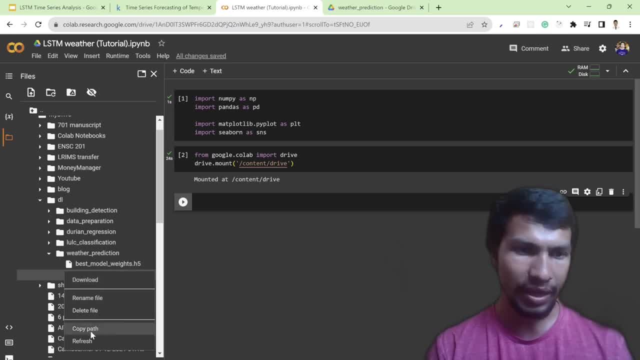 you can see that the file name is dillyweatherdatacsv, and so after that you can see that here is my data and then I copy my file path and then I'll write data path equal to and then the path and, if I like, create the data frame with PD dot read. 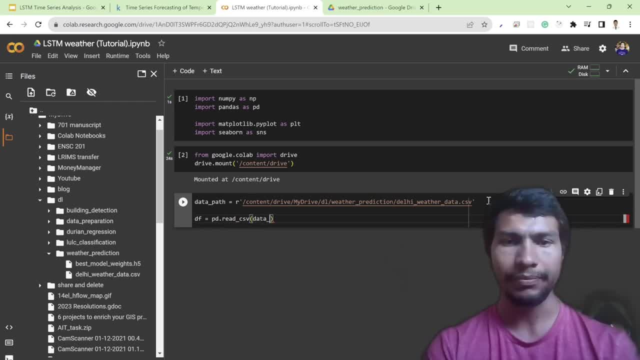 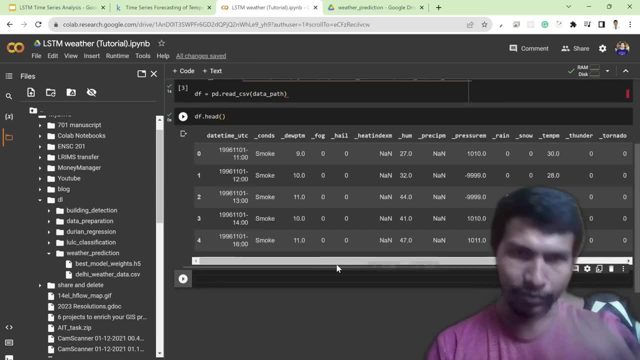 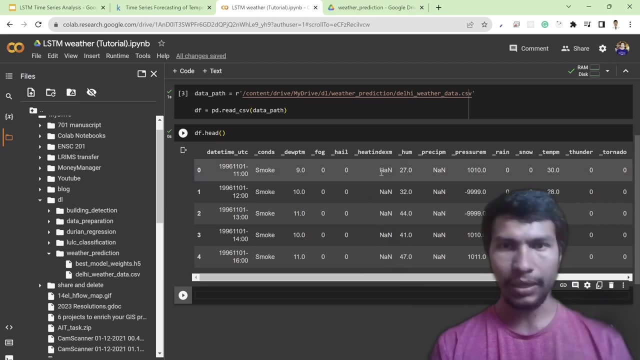 CSV and then data path and you will be able to see the data set. so here we will also see the data set below. so one thing I noticed in the actual that CSV file is like in these particular columns there are like some extra spaces, so I'm going to remove that species. in order to do that, you can write the aft. 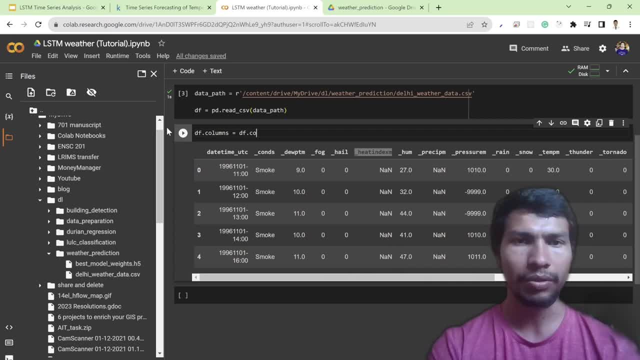 aft columns equal to df. dot columns: dot�재lhbhtrinstitshpinstituht ultimate data choice class and I'll class: quieren no de Jamesu this part. I'll request column of stier dot l sti P. so it will remove the API, not Teka generalize column if we click the. 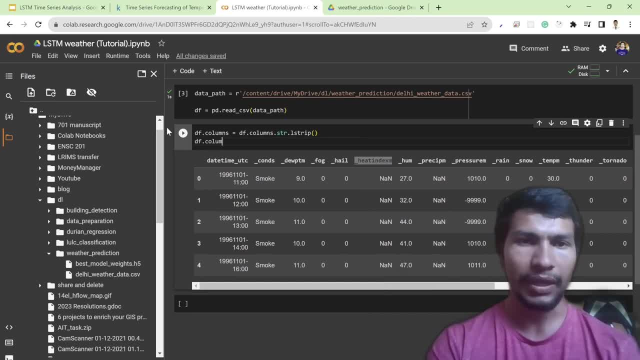 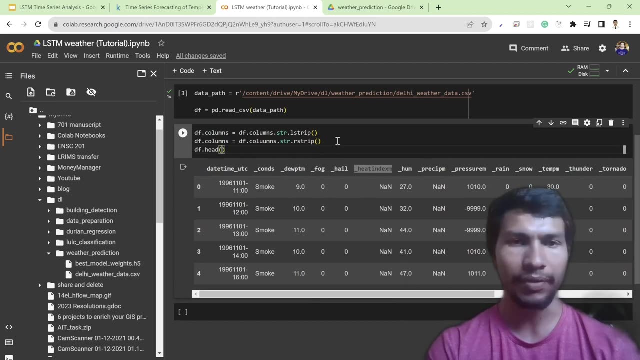 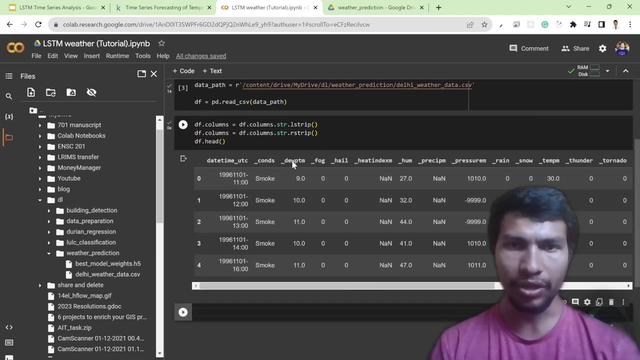 beginning, and then again you can write dot r-a-s-t-r-i-p to remove the back backward space, and then if you write df, dot head, then your result will be similar. sorry, then your result will be similar, but this time you already removed the like extra spaces. 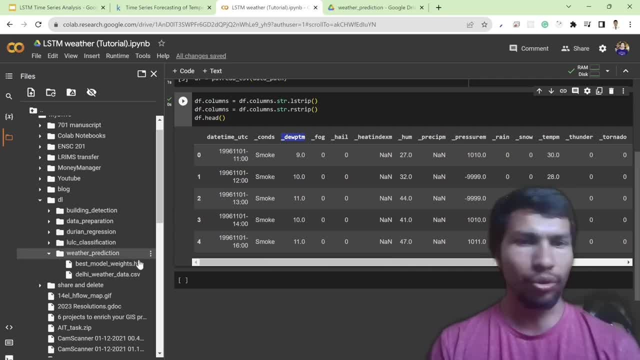 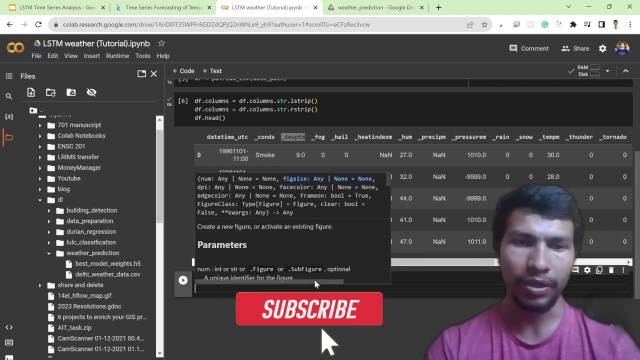 from the columns. okay, so the next step is to: i'm just going to like show you how scattered is your temperature. so, in order to like plot that temperature, so you can write plt, dot, figure, and then, uh, you can write: the fig size is, uh, i need bigger one, 15 comma, 10, and then you can write: 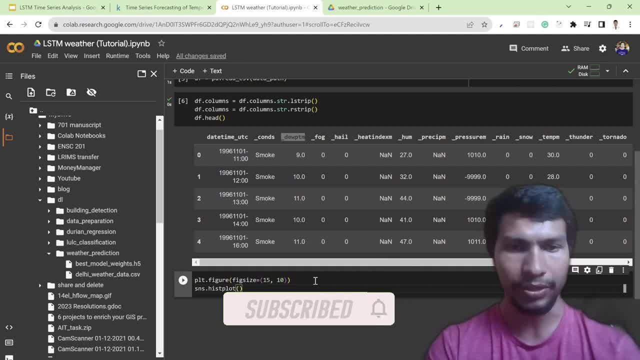 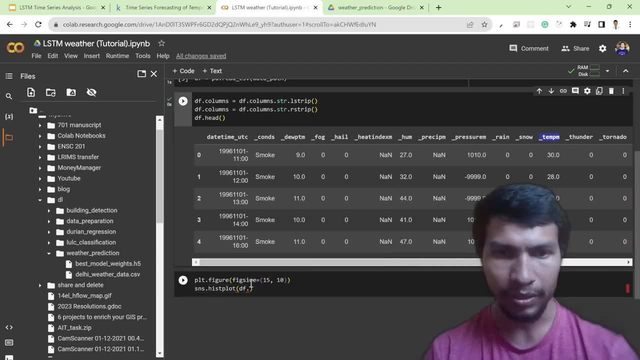 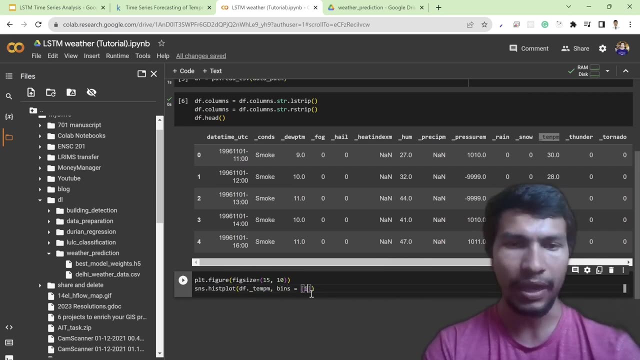 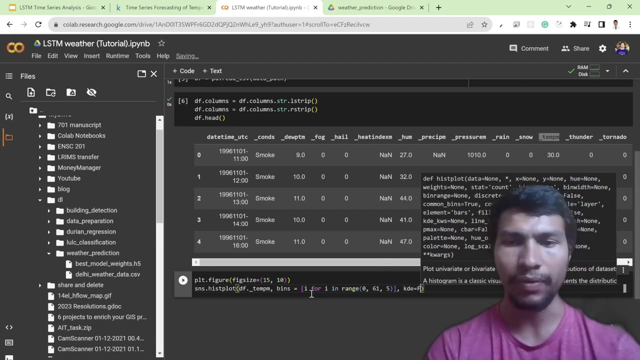 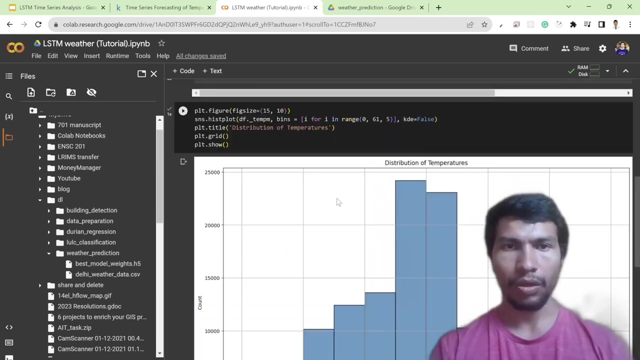 uh, you can create the hist plot based on df dot. uh, my temperature is this one, so df dot based on this property. and then, uh, your bins will be like i for i in range zero and 61 and five, and okay, kde, equal to false. all right, so this is the like distribution of 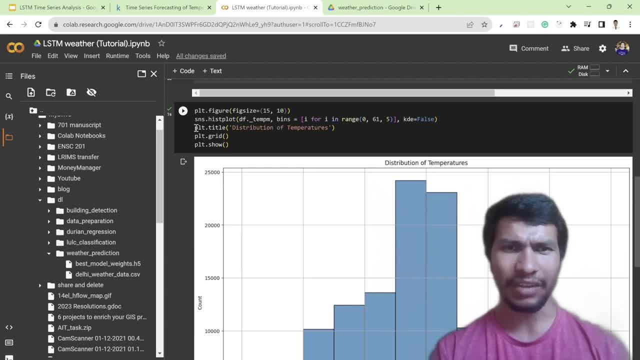 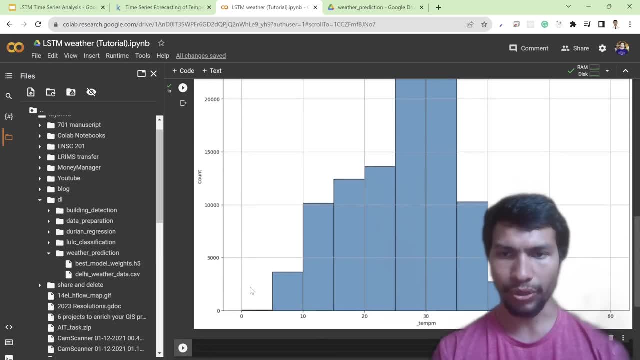 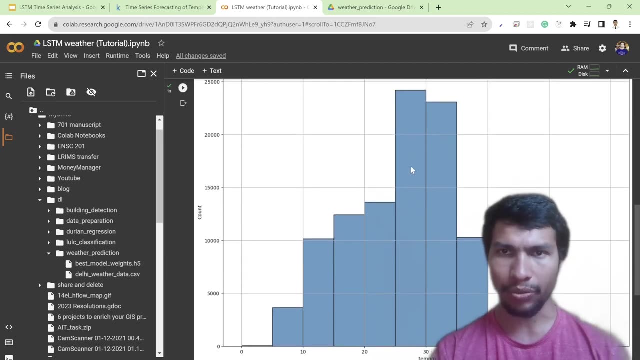 temperature and then uh, these are like totally optional things, so you can write the title and then this grid box and plt, so to show your plot, and this is the temperature value. so i, i think all most of the like temperature value lies between 25 to 30 and uh, you can see it, uh, from 30 to 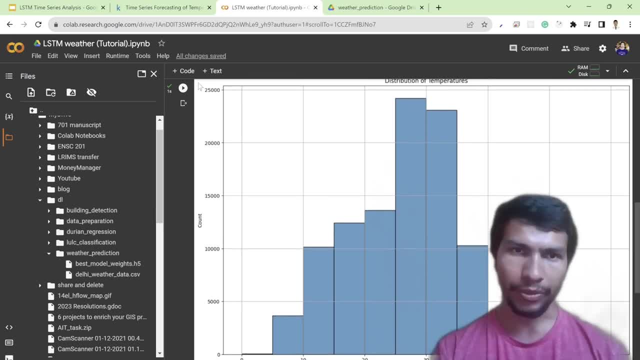 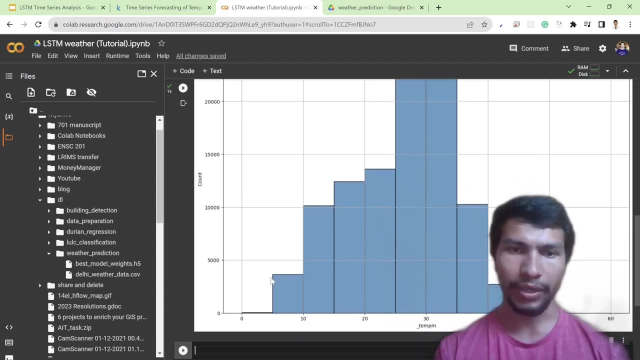 35. also there is like high value, almost around 25 000 uh temperature values lies between these two uh category and also like almost the temperature is starting from like five to ten degree in the lead. there is like below five degree. there is like no temperature below five degree and the 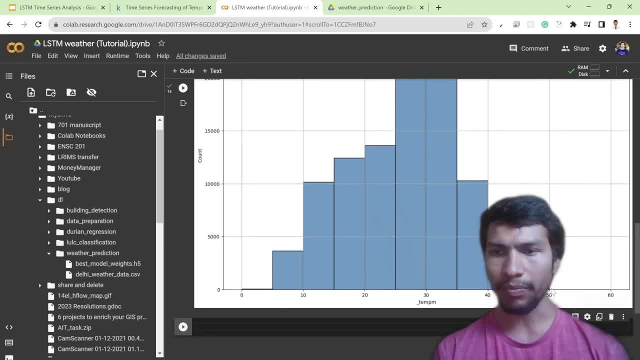 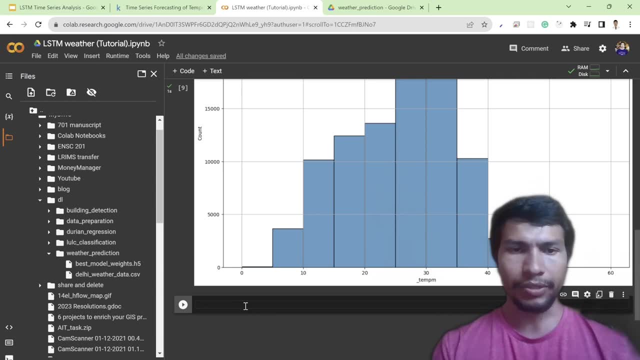 no temperature below five degree. and then, uh, no temperature above 50 degree. uh, of course it's centigrade. all right, so now it's time to like set the index of your data frame. so i'll write pd to data date time. so, since i'm using the temporal data set, so 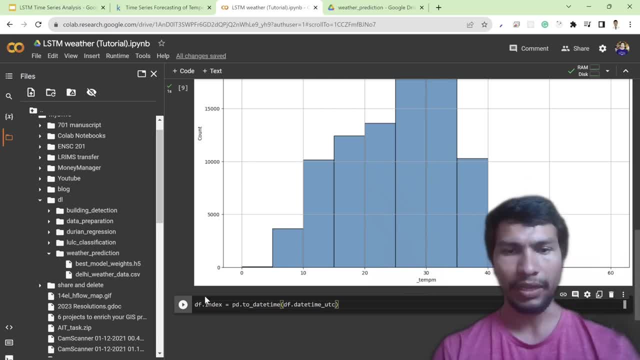 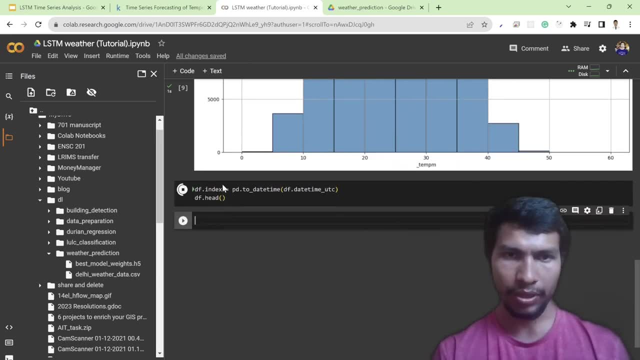 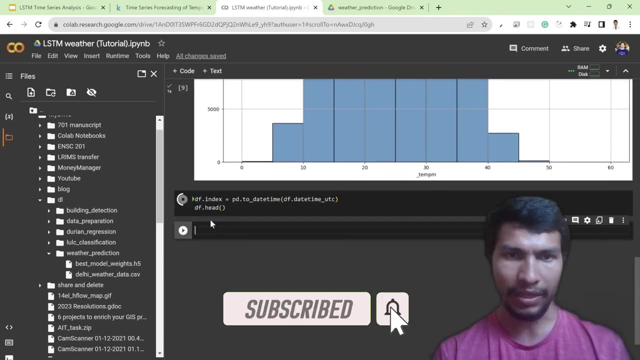 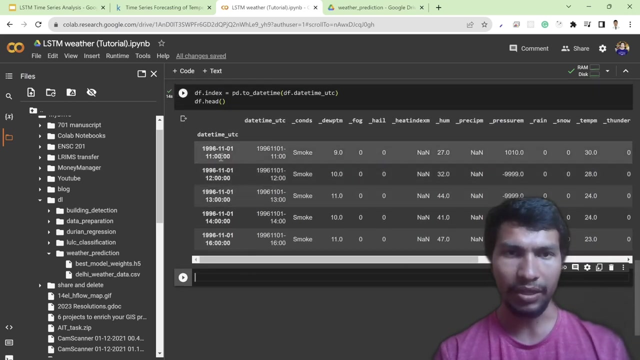 i'm going to make it uh like date time index here. so previously i have like: this index is zero: one, two, three, four. but this time i set my index is like the actual date field, so it might take some time. but yeah, here you can see that. so 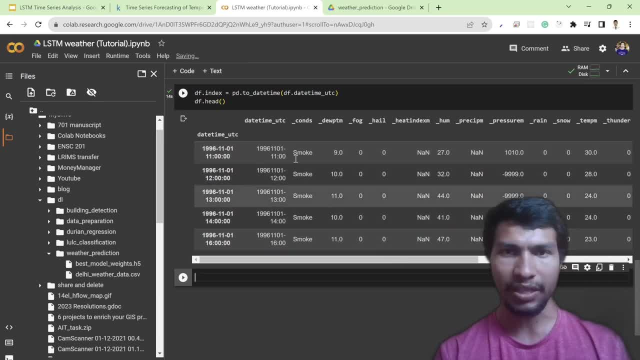 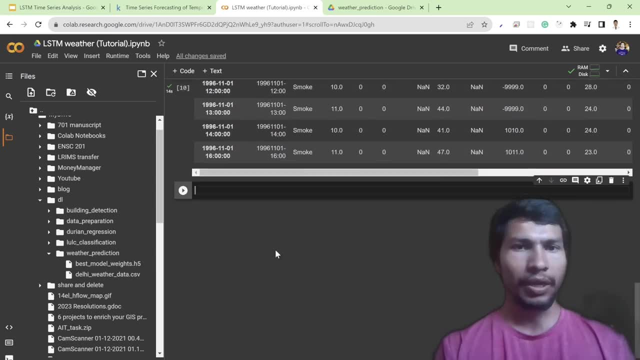 actual. my uh date time index is lies here and then these are my column names and of course you can see, and their column name is date time. you can see. so date time, utc. and right now i'm going to like copy few line of code from my previous notebook and 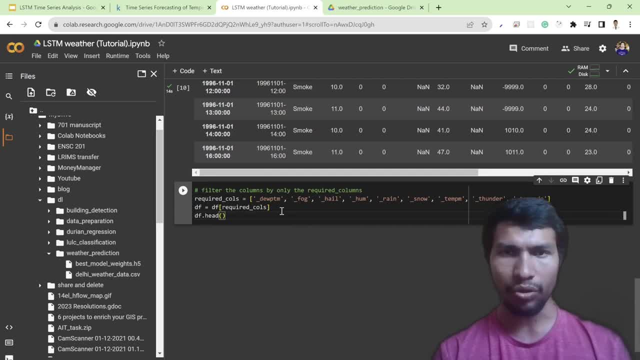 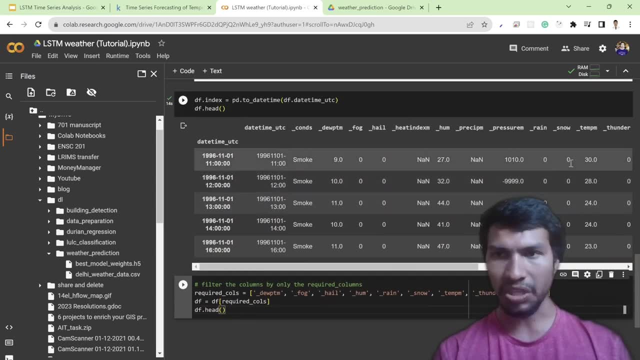 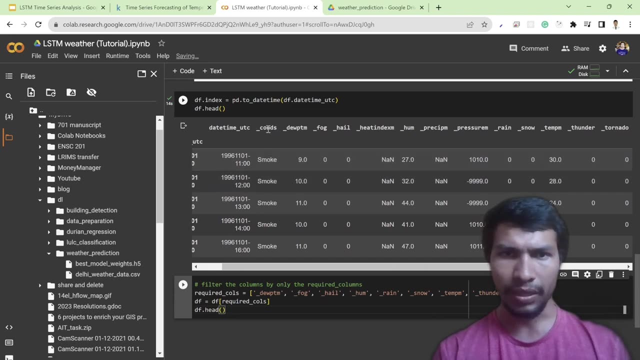 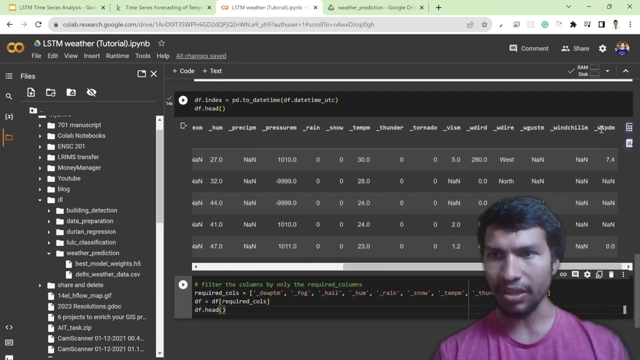 i'll explain. so right now, my required column will be like: dew point, temperature, fog, hail, humidity, rain and uh, these, these, few of these columns. uh, i, i simply want to drop few of the column, like, uh, the cons and then the pressure, yam, and uh, maybe the wind direction, uh, something. so i, i simply drop that columns and then i as i, 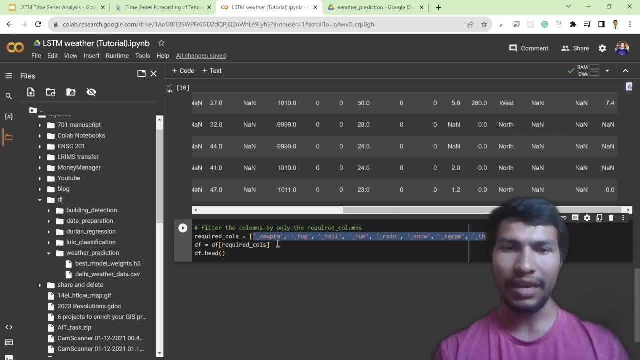 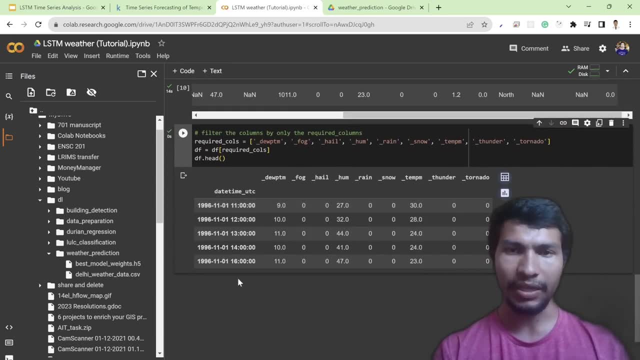 mentioned in the beginning. so i'm going to use only nine variables. so i simply filter it and then, if i see dfhead, then i can see only the nine columns. all right, so now it's time to like check the uh number of non values in each columns. so in order to do that, you can write dfisNoneSum. 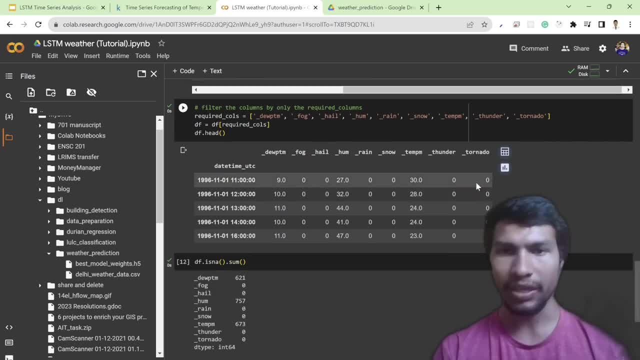 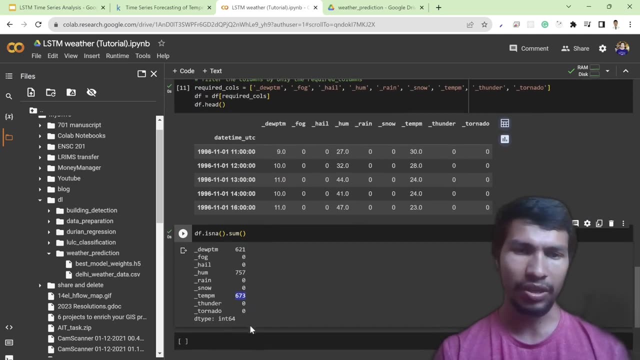 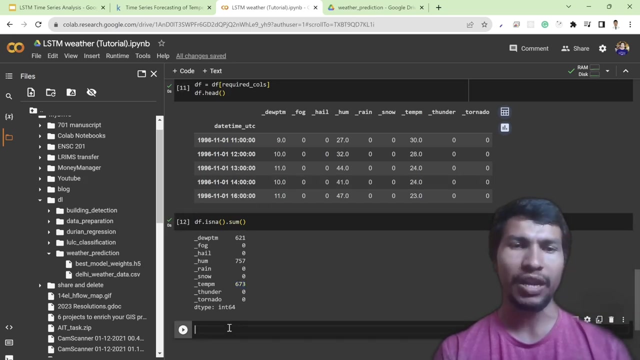 and then it will list out the number of non values in each row. so right now i have like dewpoint temperature, there are like 621 values which are none, and humidity 757 and then temperature 673. so, all right, what i'll do in this case is like i i'm going to like fill those none value based on upper must. 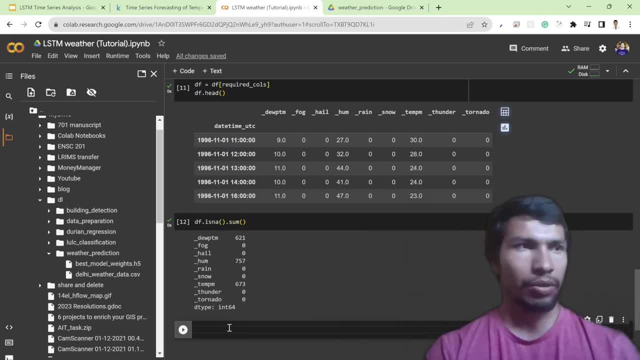 value. so. so in order to do that, so i can write dffillNone. and method equal to f, f, i, l, l, which means a fill from forward. so if i say dfhead, it will be like similar, but this time my none value will be like this, so i can write like that. so, in order to do that, so i can write dffillNoneSum. 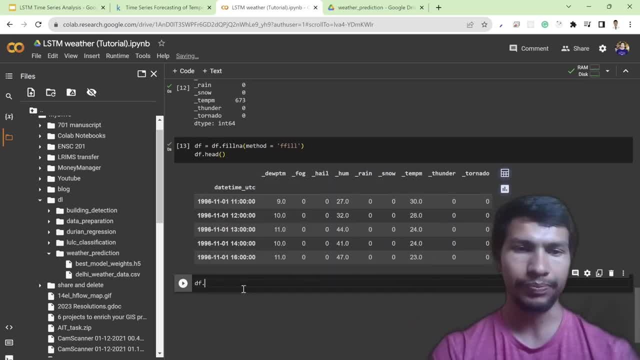 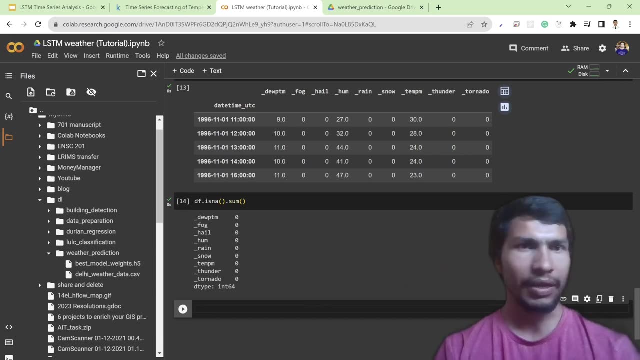 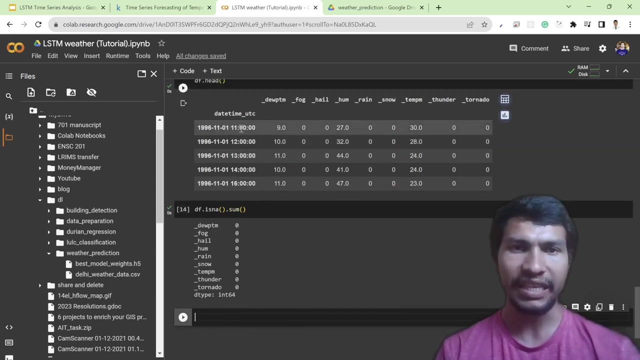 will like: go is none is an a and then some, so now I don't have any non values, so everything is filled. and now it's also like time to like resample these to the daily data set. since it's the hourly data set, you can see, we have the data. 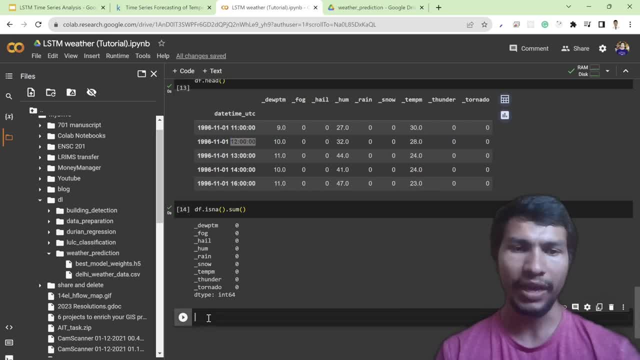 set from each hour, so I'm going to like make the daily data set in order to do that. so the it's it's very easy with the temporal data frame, so you just need to like resample it by day. if you write D, it will be the day, and then you can. 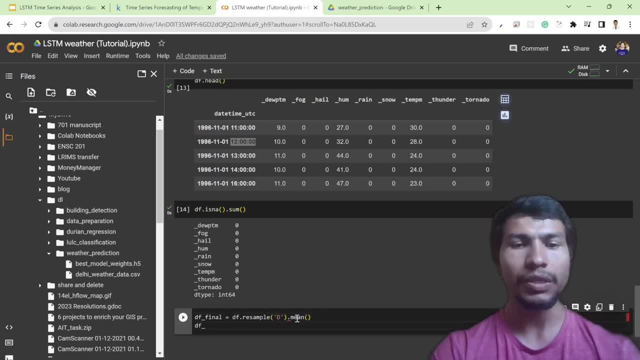 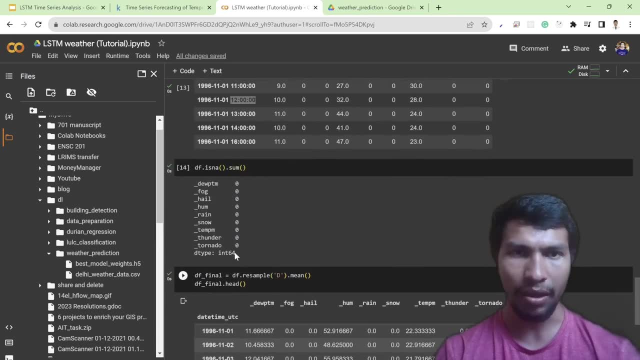 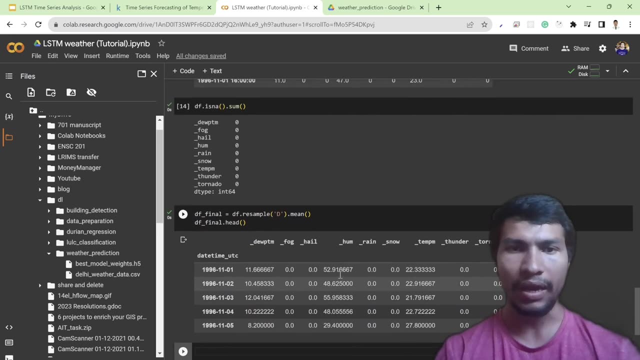 write the mean. that means you are going to every sit, and then if you DF dot here head, then you'll see we no longer have this hour, so we have only the date, and then these all values are like resampled based on day, and then these are the mean values, if you. 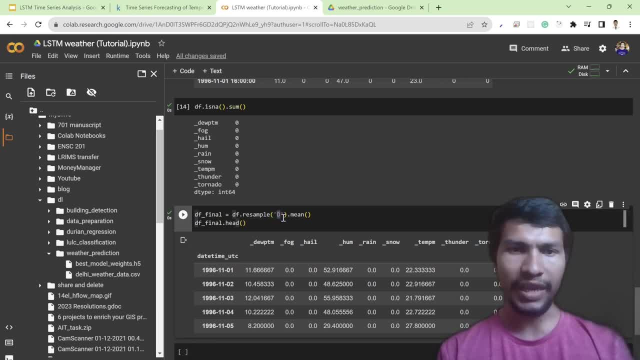 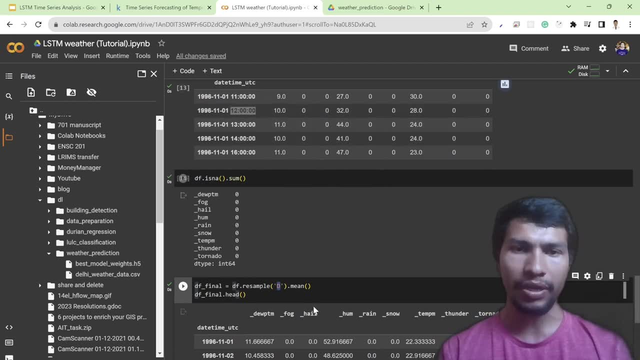 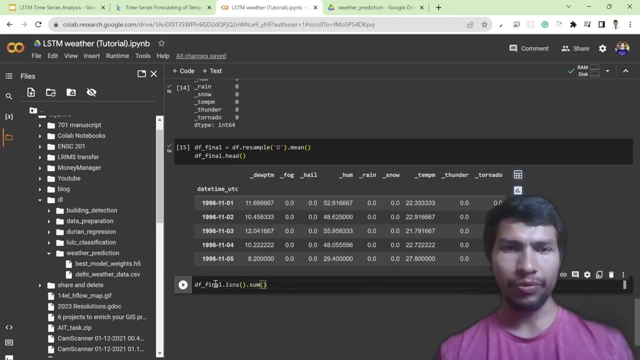 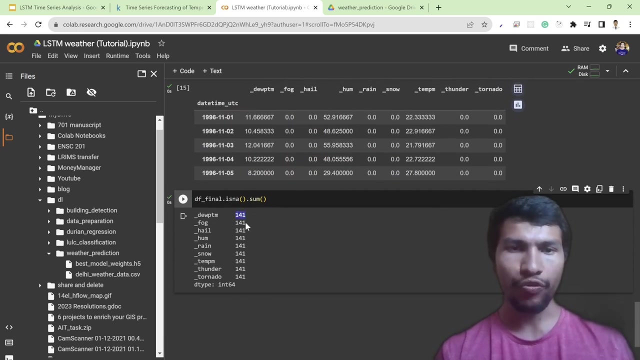 want to resample it by month, then make sure you write m, and if weekly then w, and if hourly then as since we already have hourly datasets, so that doesn't make any sense. now again, it's time to like check the non value, so here you can see all the values. has like 141 non values. 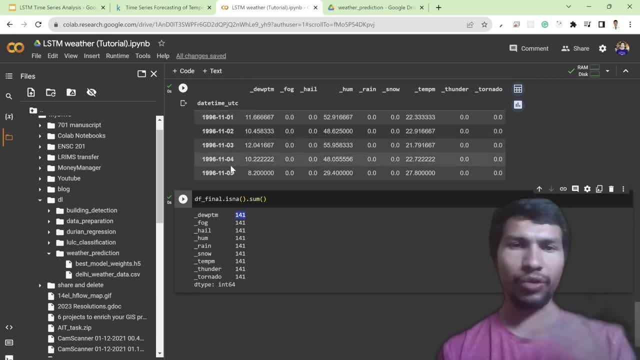 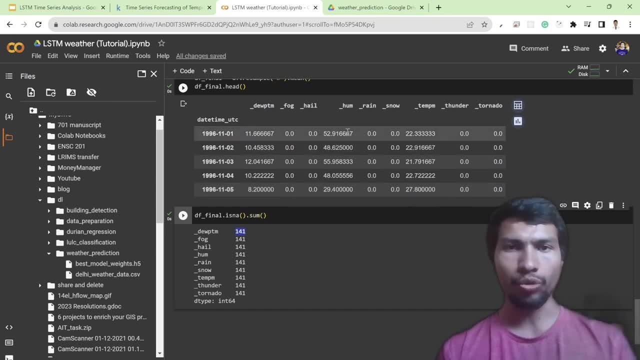 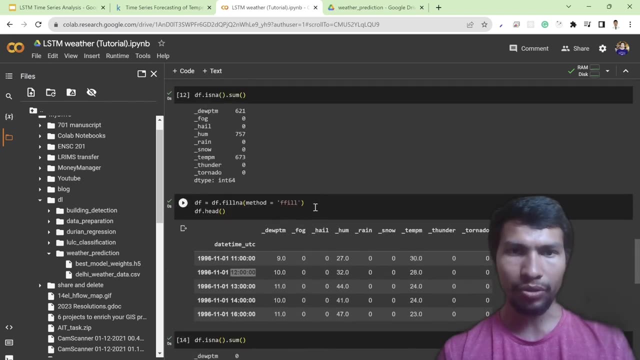 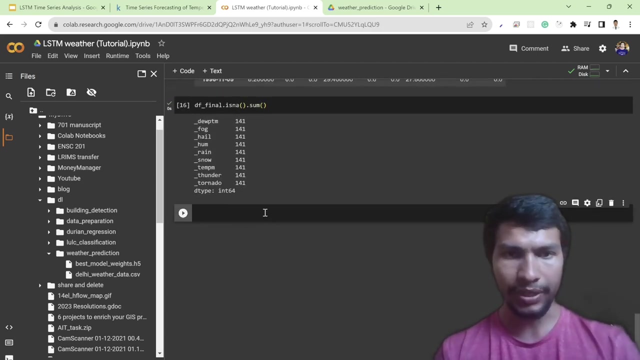 looks like there is some like missing date so, in which the weather station is unable to like detect, measure those matrices. So in order to solve that again, we are going to like use the ffill. method is previous, so maybe I can copy this cell and then paste it over here and this time it will. 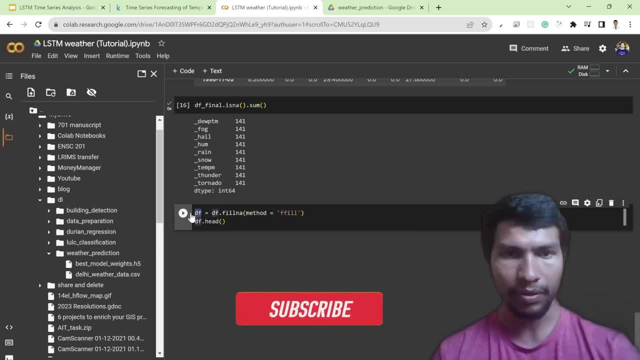 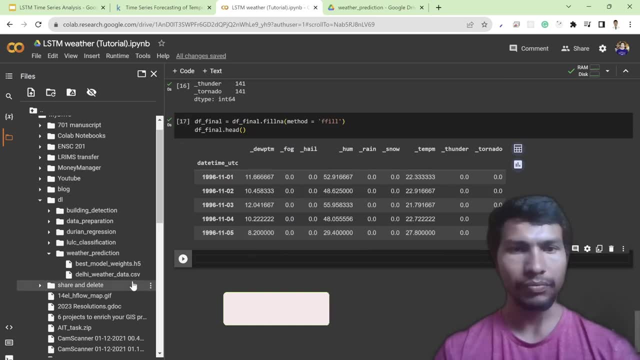 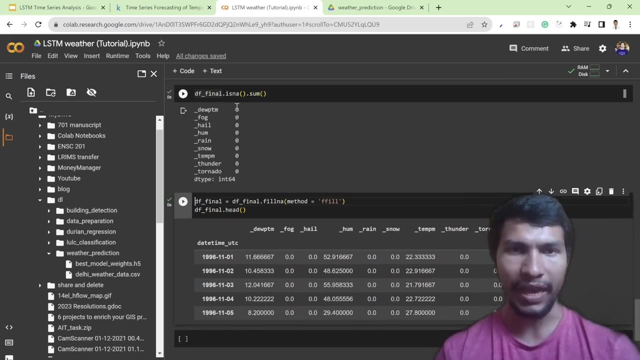 be like: instead of DF it will be DF, final. okay, now again we can take this, we can again take this cell. so now it has like all the like columns were filled by ffill method and then now we don't have that, we don't have that, missing values. 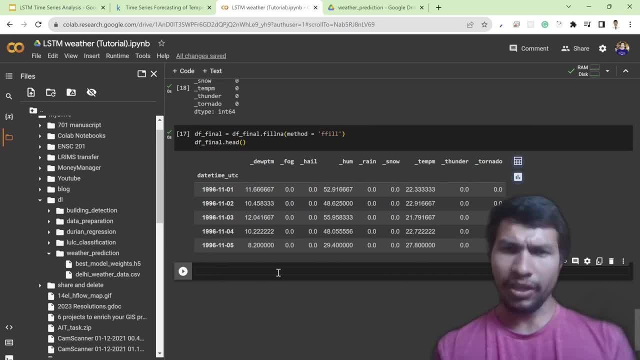 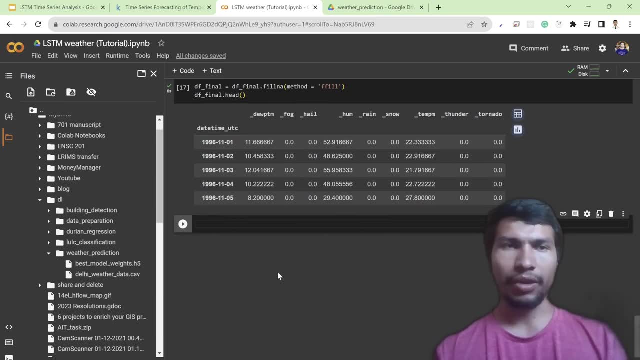 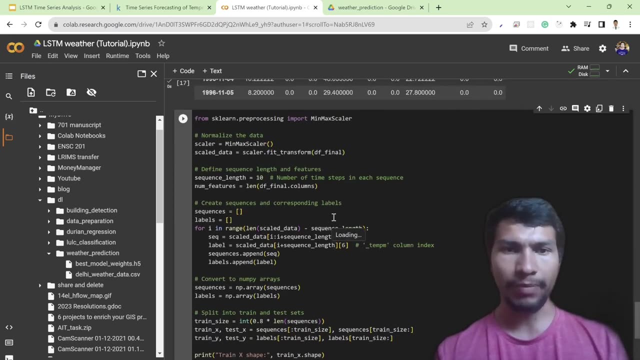 anymore. now again, in order to like make this data set in the like actual good format is like required in LSTM model. so I'm going to like copy and paste some line of code and then I'm going to explain what what's going on here. so let me. 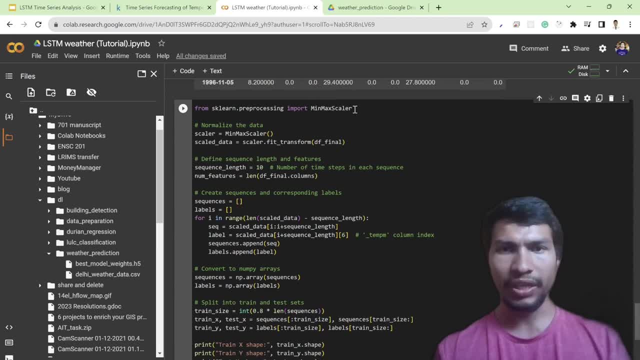 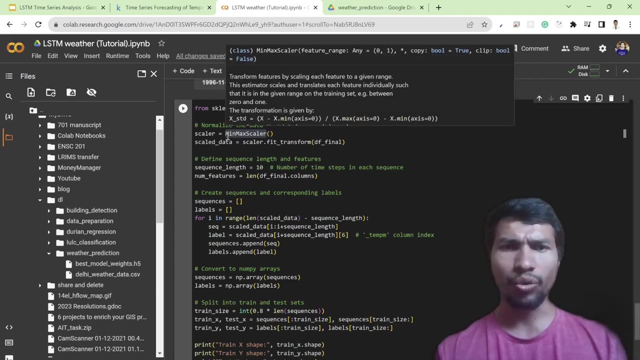 explain. so, first of all, we use the min max scalar, which is like normalization of data. so if you want to achieve the best accuracy in your model, then make sure you need to like, normalize these things, normalize the data. so what this min max scalar do is like if the like 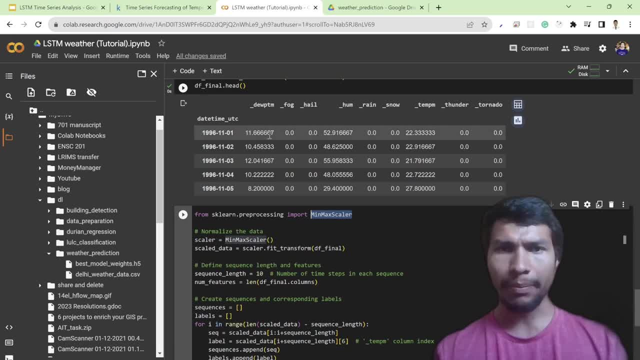 temperature. it will just take the minimum and maximum value from each column and then try to like subtract, I mean try to compress it into the value between 0 to 1, so it will relatively change all the values so that we get all the like points, all the all these numbers between 0 and 1, and then 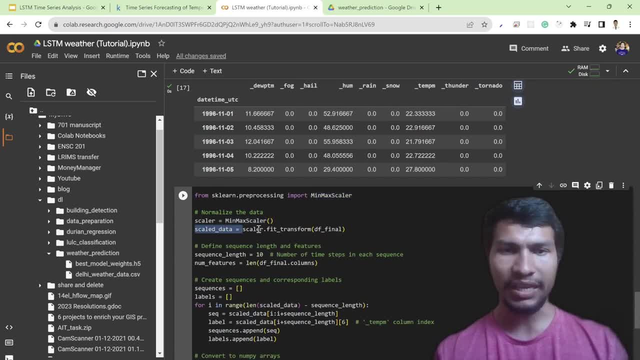 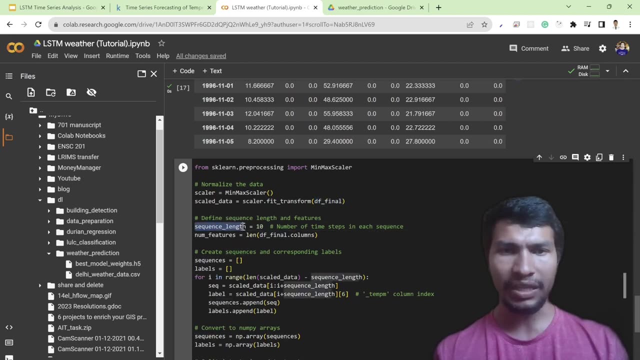 now we are doing the like: a Skeldata is the same scalar, and then we are like scaling everything in the DR final, which is over here, this data frame, and after that we are trying to like make the sequence length of 10. that means it will. 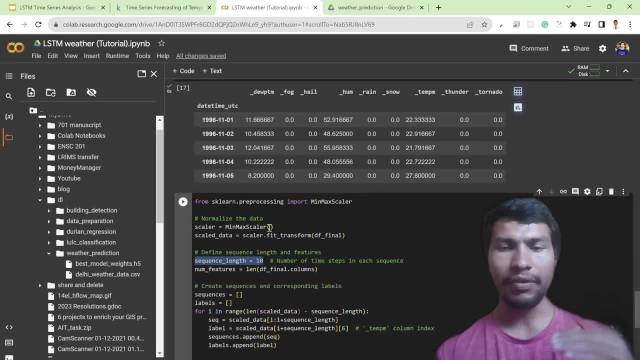 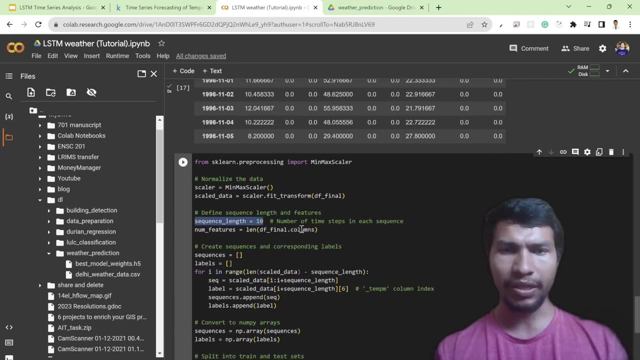 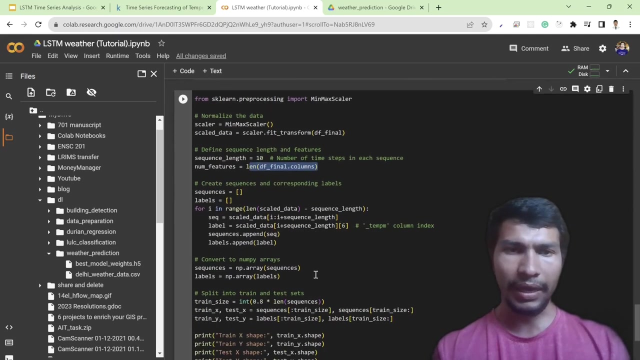 take all the variables from 10 days, from like previous 10 days, and then it will try to make the sequence of 10 days and then try to predict the 11th day, temperature. and here our number of feature is their final dot columns. of course you can replace it by 9, because we have 9 columns and here I'm creating. 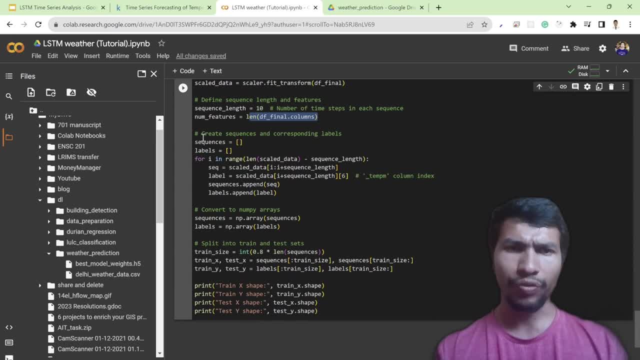 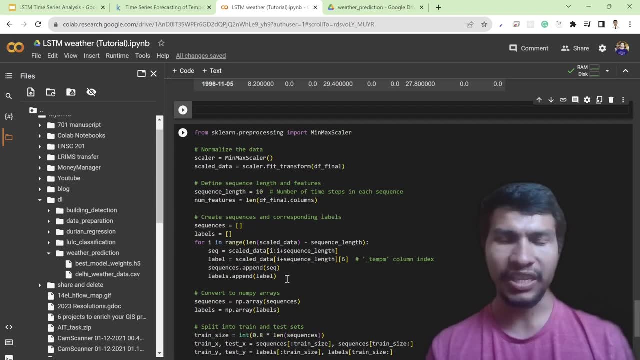 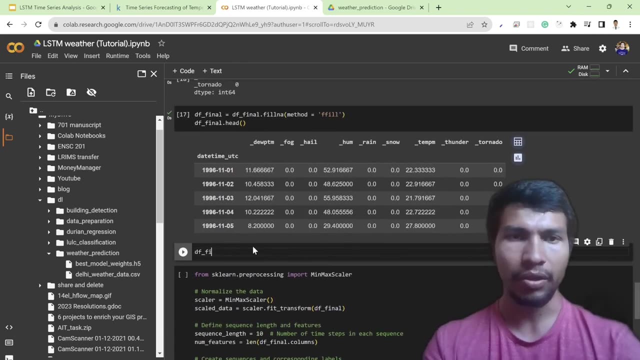 the sequence and corresponding labels. so first of all I create the like empty list. this loop here is the most trickiest part and then this is the most essential part. so in order to explain that, I am going to like again print out the my data frame dear final dot head. this time I am printing, I think, around. 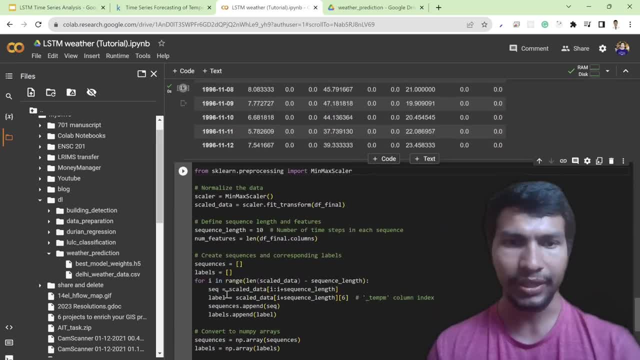 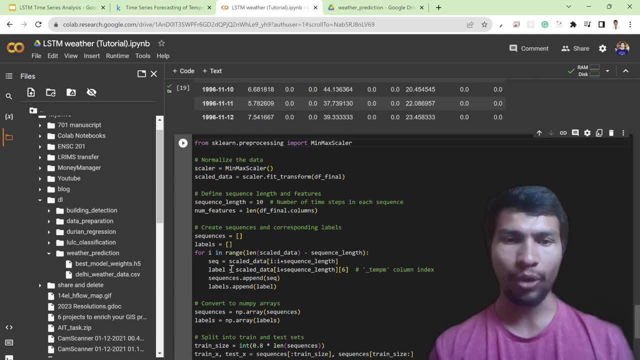 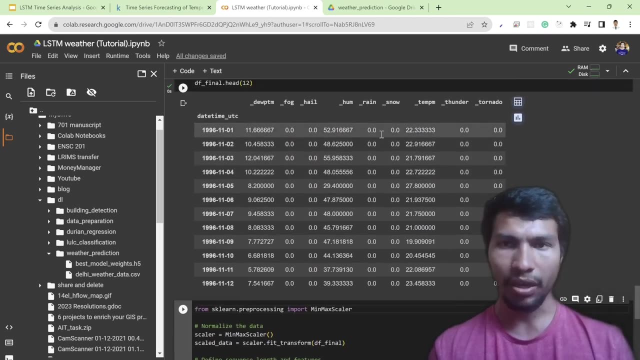 12 data set. so yeah, so here. so from this loop, what it will it is doing here is like it, it's creating the sequence and the label and here, for example, our sequence will be like the: all the variables from up to 10 days, even containing temperature data set. but 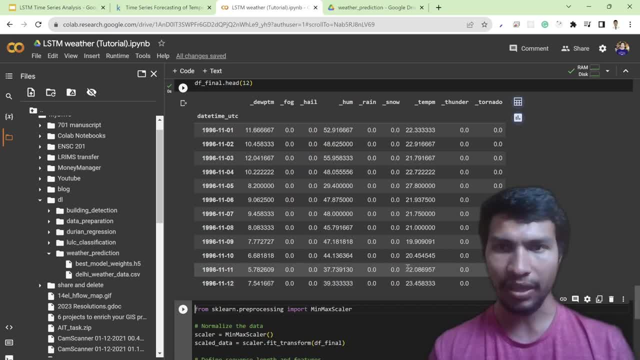 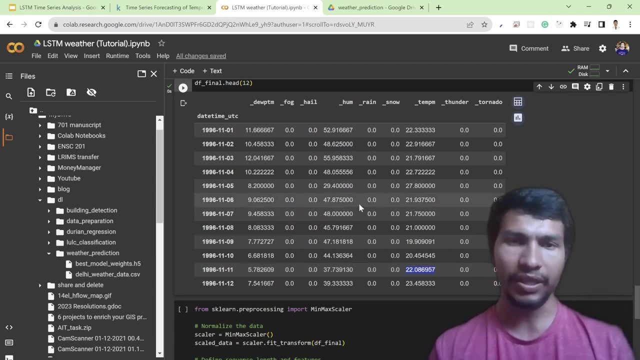 our like label will be the 11 days temperature, which is 22.086 degree centigrade, and then we are going to create the sequence and then we are going to then, for the second iteration, it will take all the values from date 2 to 11. 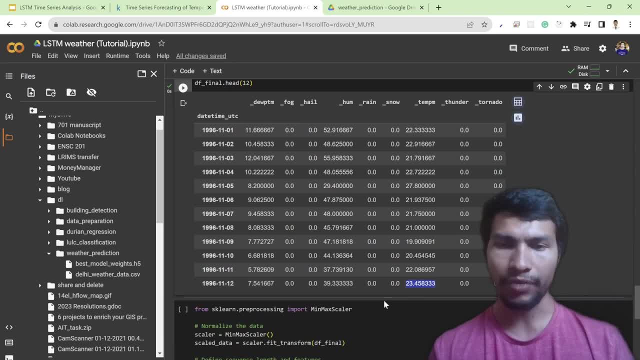 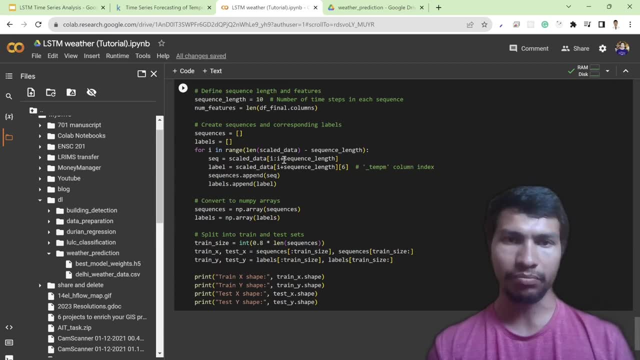 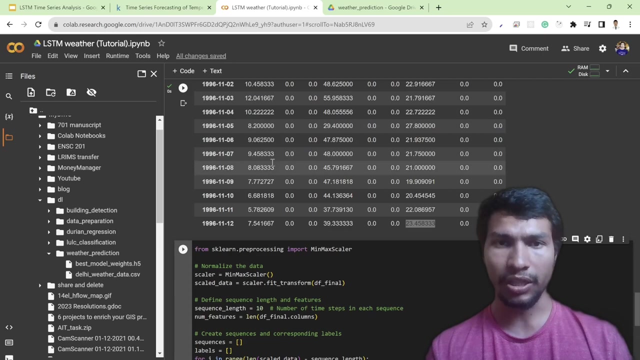 and then our predicted level will be 23.45. so that's what it's doing here, so you can like simply read it. it's explained here. so I'm here. in the second line, I'm taking the sixth variable, which means like index is here, starting from 0, and then it's the temperature: 1, 0, 1, 2, 3, 4, 5, 6- and also like: 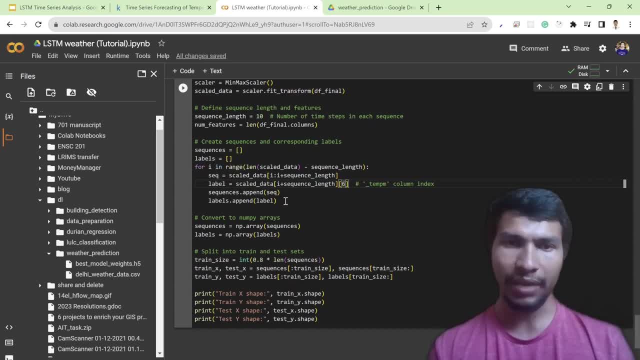 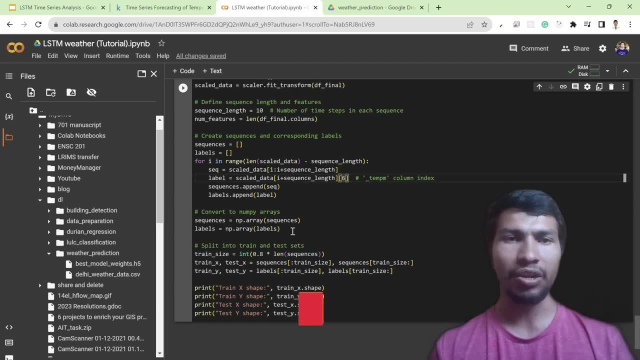 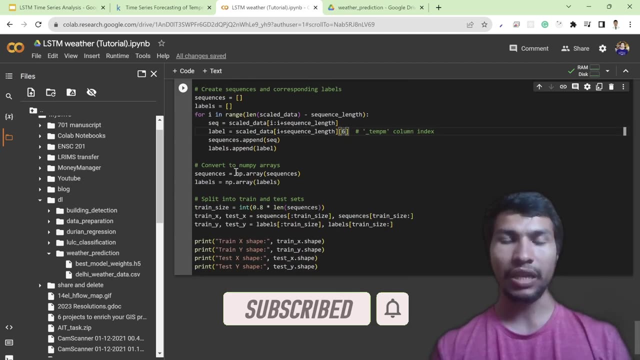 simply after like creating my sequence and label, I am appending those to the list and then later I convert them to the numpy array. in order to like train deep learning model, you need to like pass. it is a numpy array or pandas data frame. that's how. that's why I created numpy array and here I am going to like. 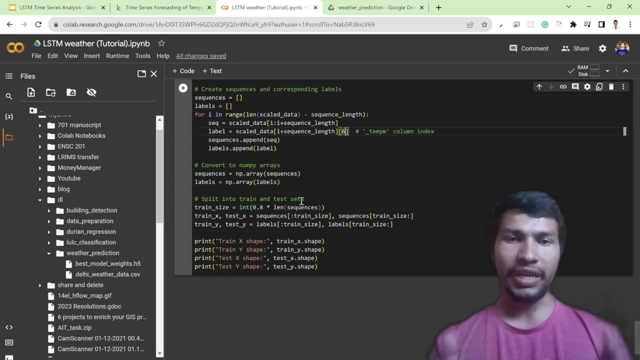 here I try to like split the training set and test set. so I'm like simply splitting them based on 80 to 20 ratio, and here I simply selected: the first 80 percent of my data is the train set and then last 20 percent of my data is the. 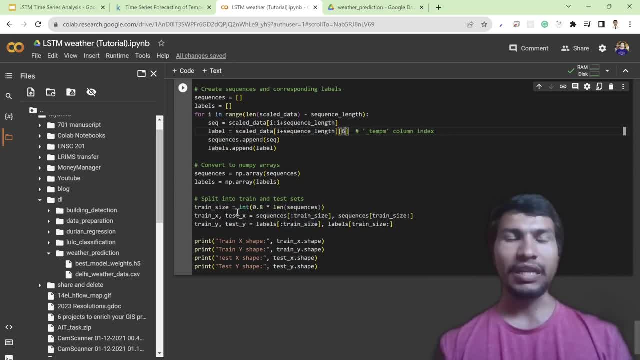 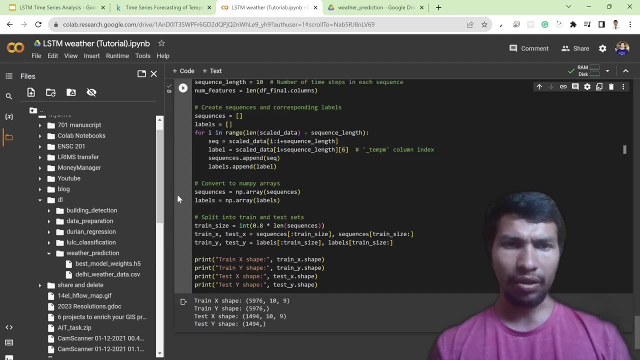 test set. that means these are of course the date, time index, time series, data set. and then I'm like simply printing my train X and train Y, test X and test y values. so it might take some time to like run, but I think it's quite fast. so 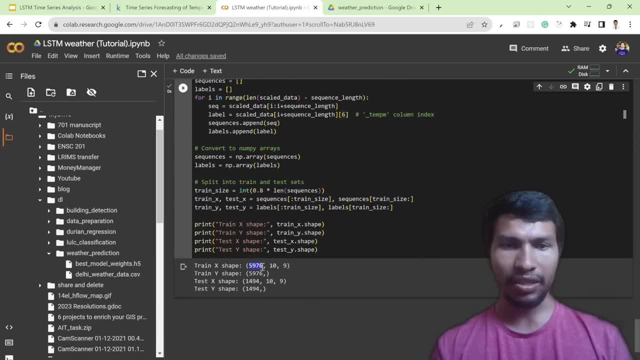 here you can see, we have like this, much of like delegates it, but we have the like 10 sequence with 9 variable, and then our level is all the like. based on this trainification and 9 variable, we have only one value: is the prediction, which is, of course, the. 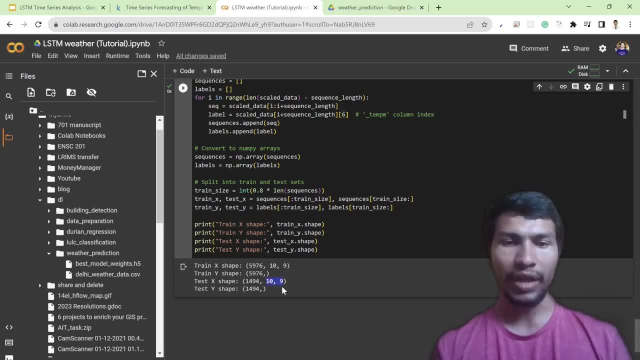 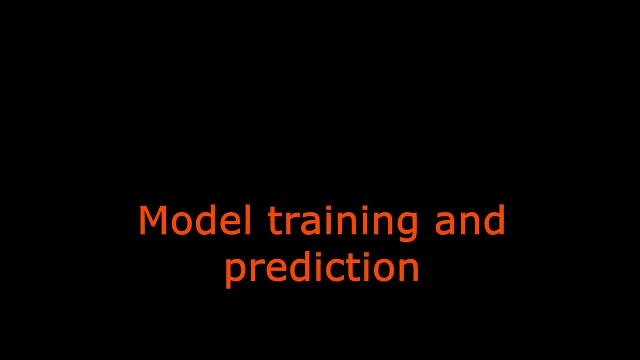 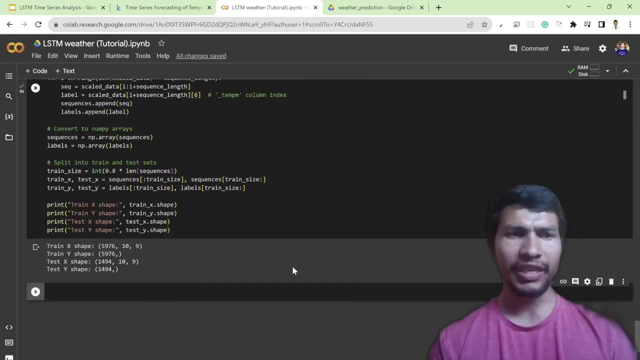 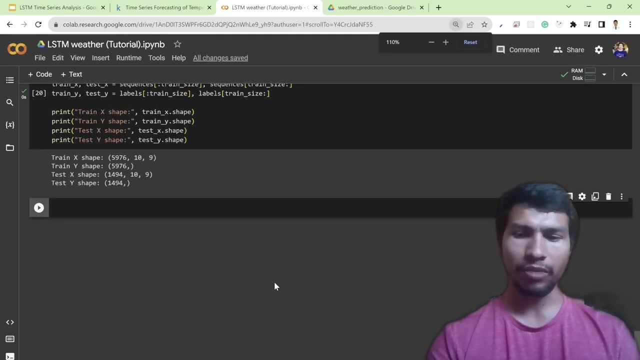 temperature, and then here also we have 10 to 9 variable and then of course we have like one output is label, all right. so the another important thing is to like create the model. so, in order to like create the model, so there are like lots of options so you can search. 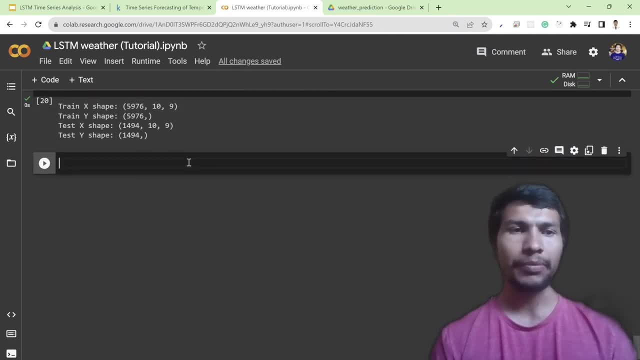 for the open source, any like github repository, or even you can ask for the chat GPT. to be honest with you, I also asked for this particular model in the chat GPT and then I try to like adjust some of the parameter. so that's how I. 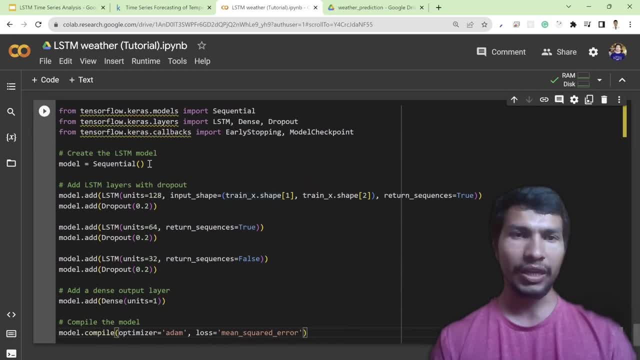 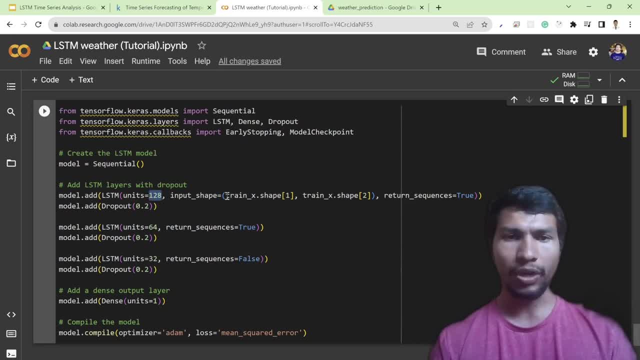 beginning unit and input shape will be like my shape of my data set, which is like 10 comma 9, and of course, I need to like pass this important- this is the like important things here, so I need to return this sequence is true, but at the end of my model I need to like make it. 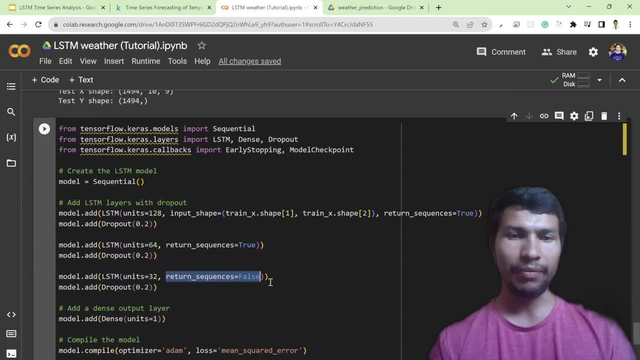 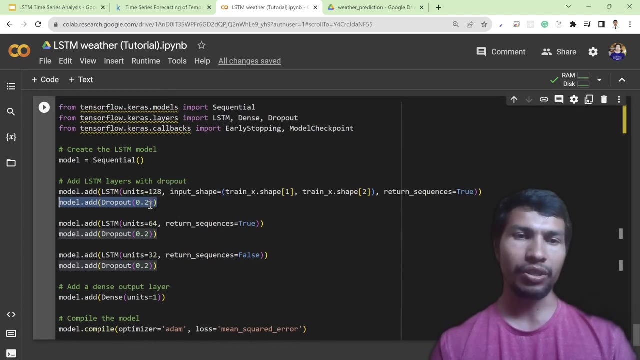 false, so that it it will be able to predict this time. otherwise, I need to like pass my sequence over and the LSTM model, and I'm using this dropout function 0.2, of course, in order to like reduce the like overfitting complexity. so, in order to like get the 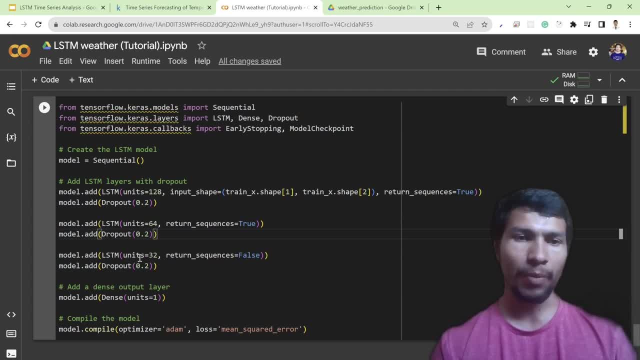 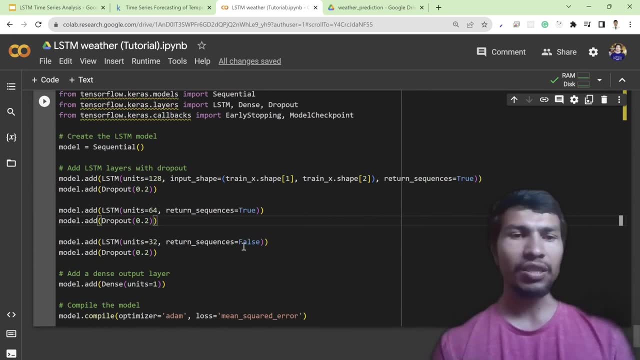 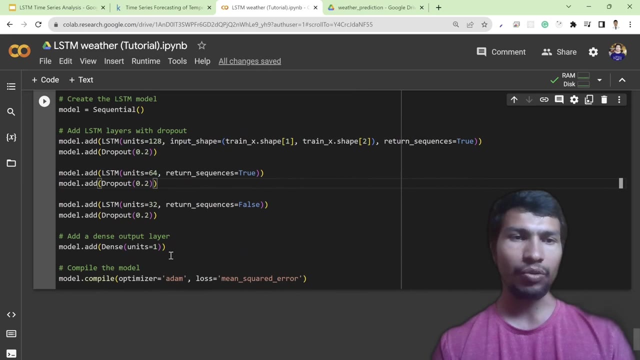 more accuracy, so I added three dropout functions. of course, it's up to you. you can like modify this model or make it more like, more dense, but for now I feel like I am just trying to like detect the temperature. that's why I added only three layer: LSTM layers and, at the end, so you need to also add the dense layer. 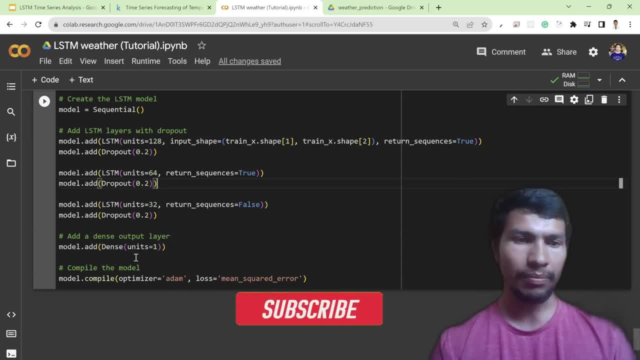 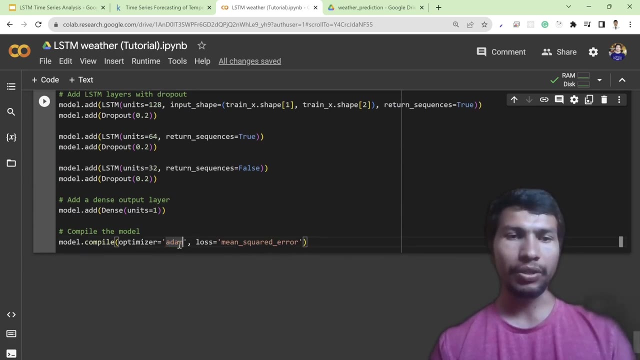 with the unit 1, which is the output layer, and of course you need to like compile it with the like optimizer. of course, as far as I know, the Adam optimizer is the good one, so I always go with Adam, but if you know any better optimizer, then let me know in the comment section as well. so 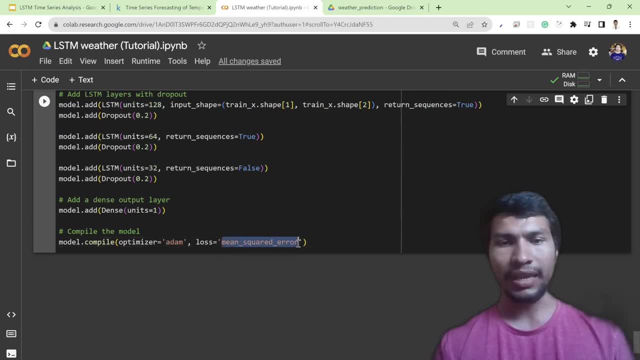 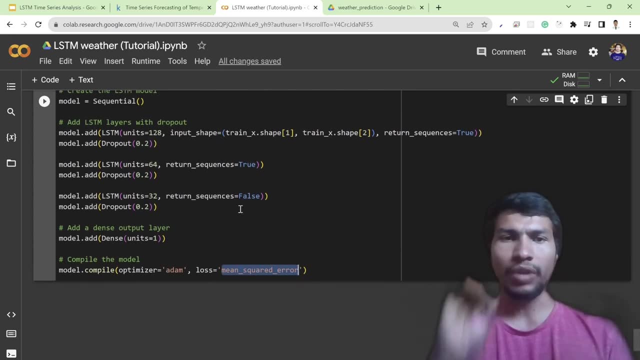 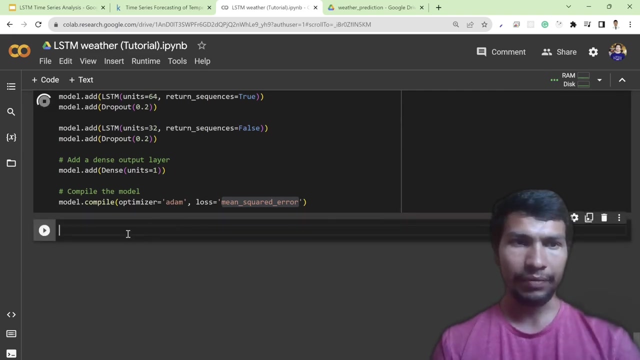 and also the loss function. is the like also essential one, since I am doing the like regression kind of problem. so I'm trying to like get the prediction, as a number is a like temperature. that's why I wrote it as mean square error is the loss function. so simply run it and after that. so if 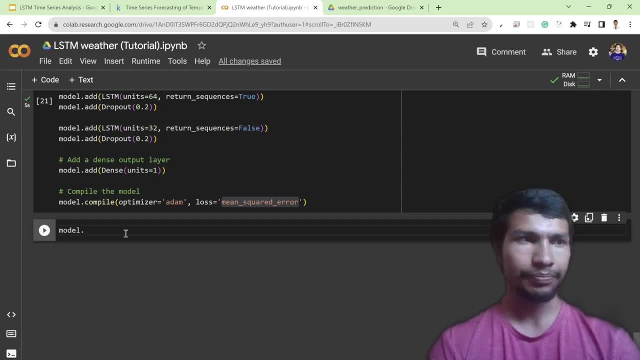 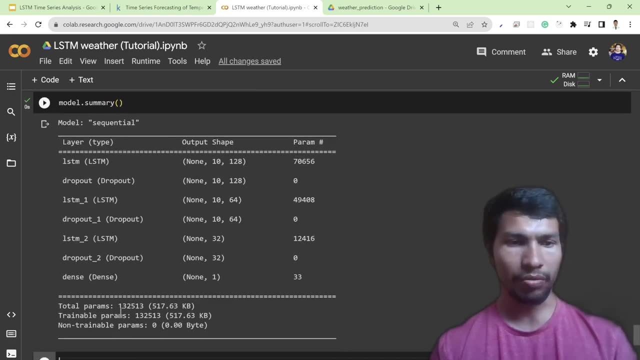 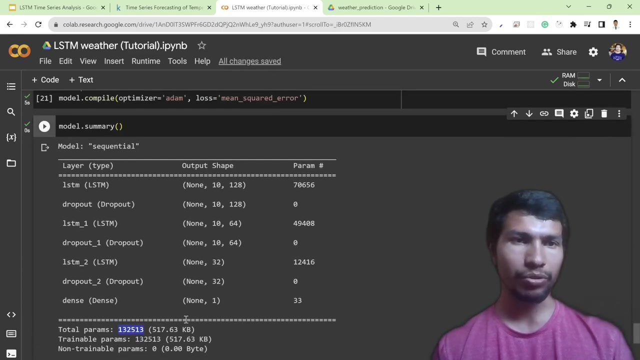 you like write the model dot summary, then you will see all the model and then total parameter, trainable parameter and non trainable parameter. of course we don't have any non trainable parameter, but it looks like I have like 132, 132 thousand of parameters. so yeah, so we need to like train this model. so now in 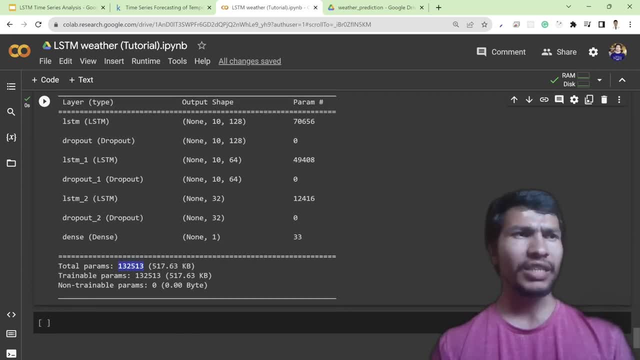 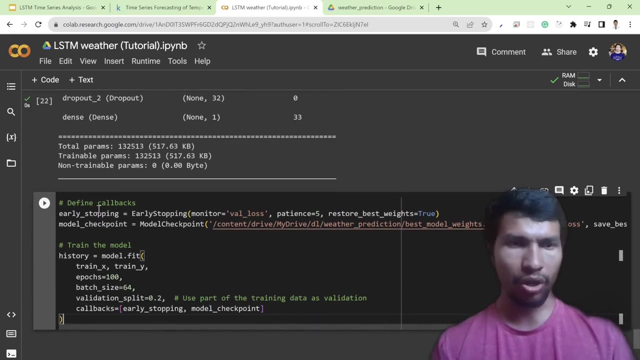 order to like train the model. so the two best things that I always try to include are like early stopping and then the model like checkpoints. so let me copy some code from my previous repository and explain here. so, early stopping, I try to like add these two callback: 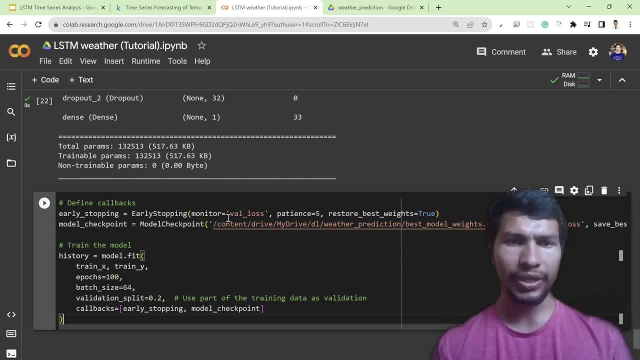 functions. so this early stopping. what it will do is like it will monitor the val loss, which is like run in the validation dataset, and it will like monitor the loss value of that that particular, like epochs, then it will simply run it till like we get five consecutive non better values. 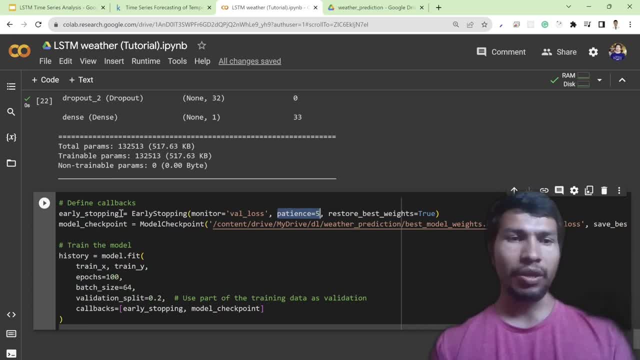 then it will simply try to like stop. the purpose of this early stopping over here is to like: save our time. if the model try goes like the, if the model went to the overfitting stage, then it will simply try to stop our model based on like five consecutive values, and then, of course, I'm restoring the best waste. 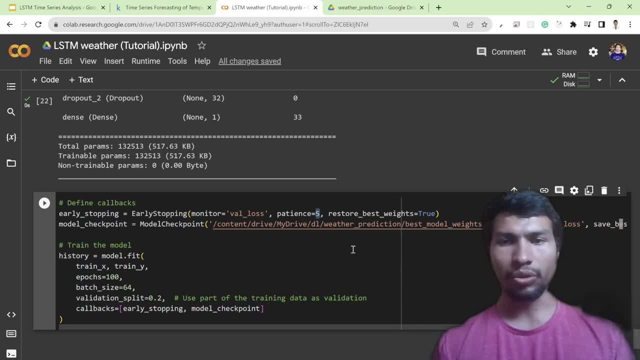 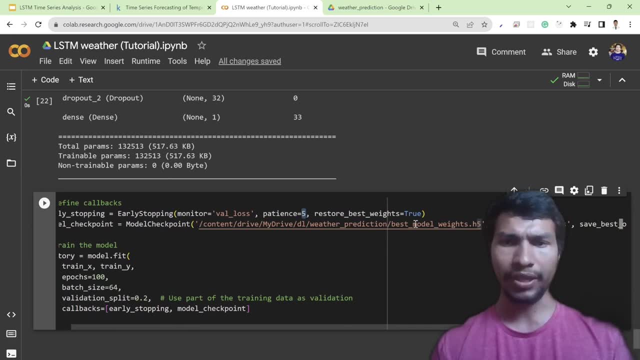 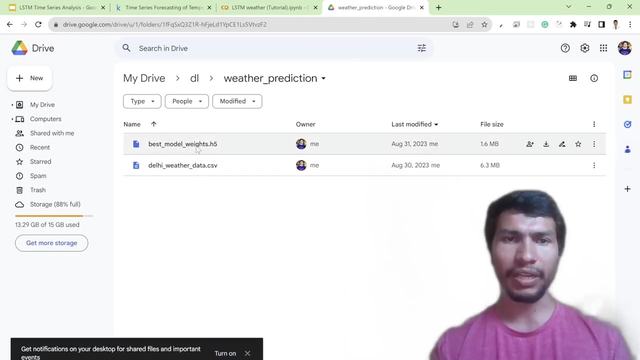 is true. and then model checkpoint. so this is to like save the best weight. so here I have the like location to the best weight function. so since I already run this function, so I have already like best model weights over here. but anyway, I'm going to run it again and 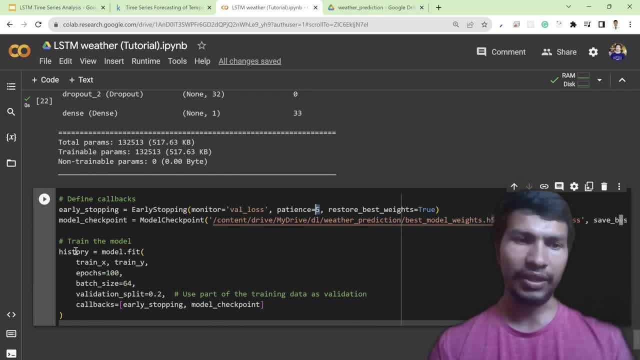 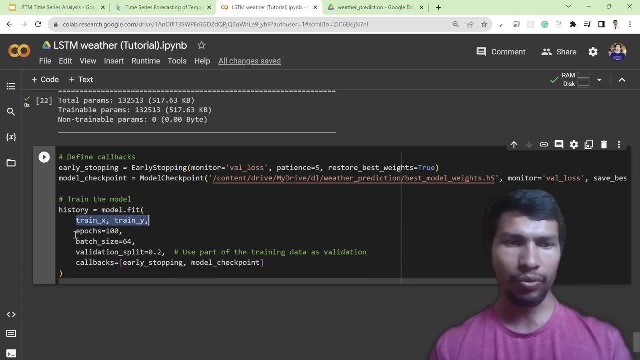 and yeah, it will also monitor the var loss and here in the history, actually during fitting the model, so i'm passing my train x and train y value and then i'm running it for like, for now i'm i'm planning to run it for 100 reports and then batch size will be 64. of course you can, you can make it smaller or 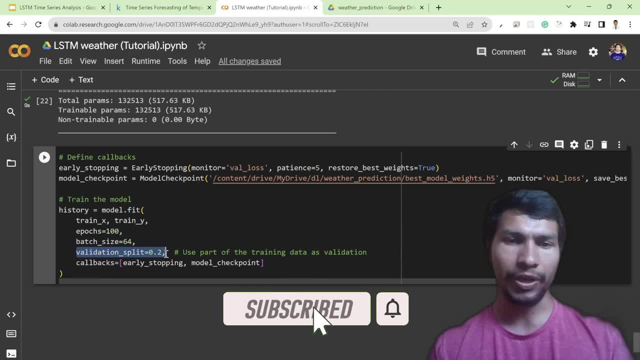 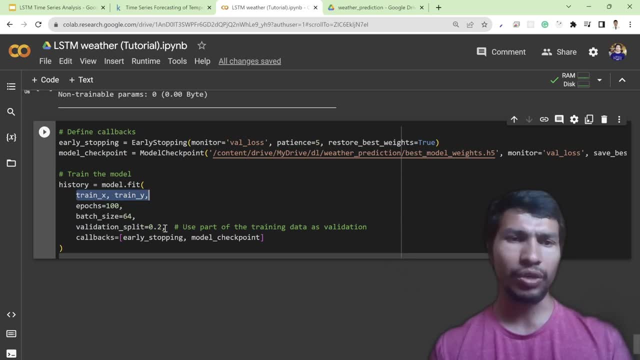 even bigger and then validation split is 0.2. so what happened here is based on, like this, train data set. so it will simply again split our training data set by 80 to 20 ratio and then, uh, it will train based on the 80 of data and then validate our model based on 20 percent. 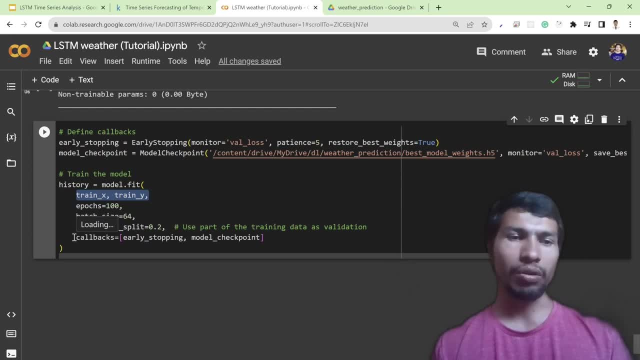 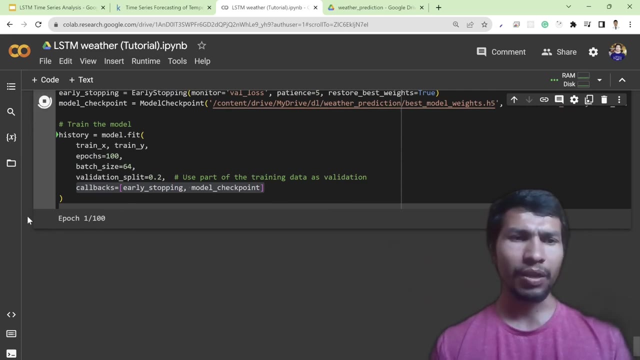 of data and then, uh, get the more like nice accuracy and then i have to call basically different in the consistency students in these videos. so basically i have a functions and let me run this and of course it will take much more time- I think around 10 minutes or something. so I'll resume the video after, like. 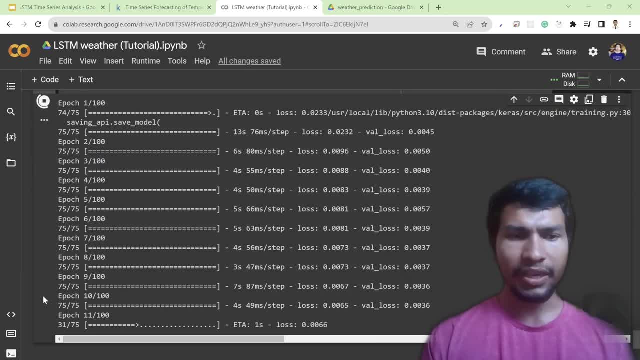 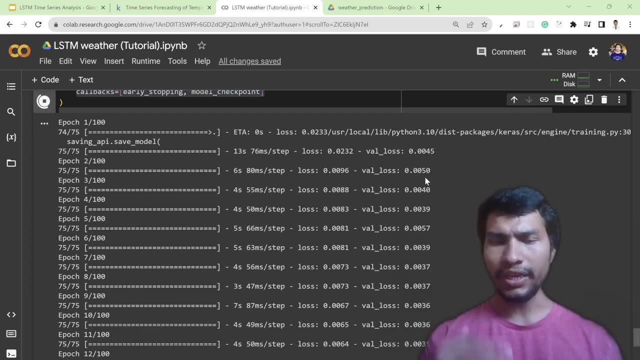 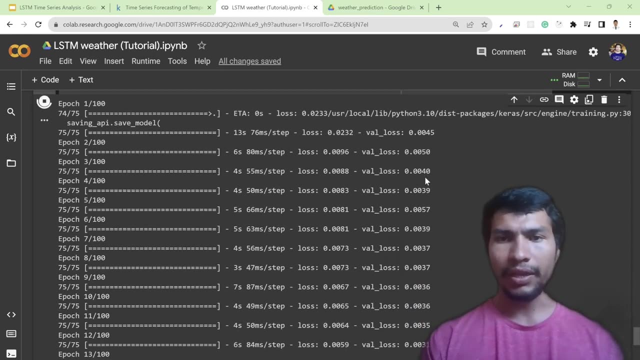 training this model. one thing here I want to explain one thing. so we are just tracking file loss. if the file loss is lower, getting lower value, then that means our model is still training and then it's doing well, and if it start like increasing, then that means it's not a good. it try to overfeed the model. so 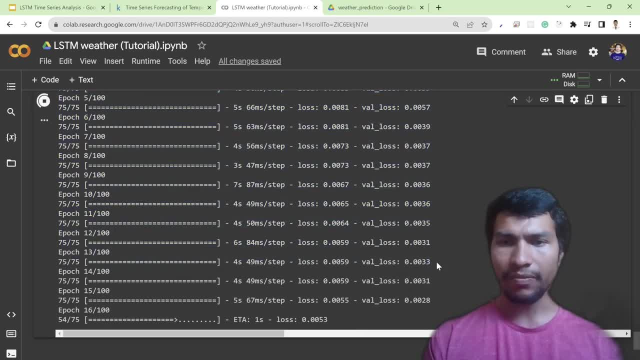 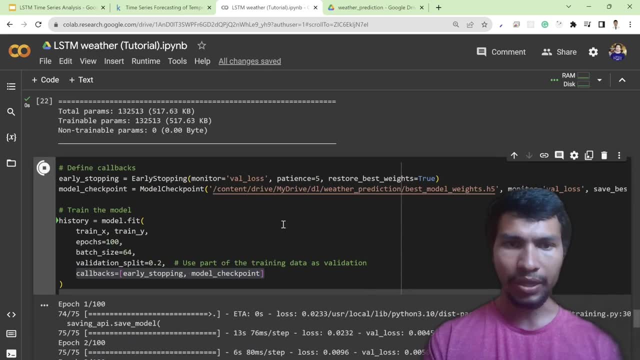 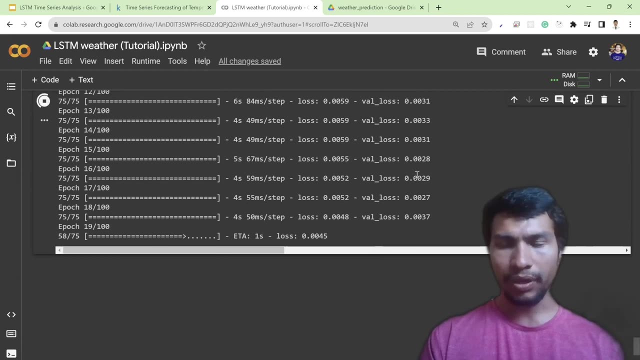 that's why I'm simply tracking this file loss function and then if it start increasing, then, as I mentioned here, we have the early stopping check pointer, which is like callback function. so if it start like increasing for five consecutive epochs, then it will simply stop our training. 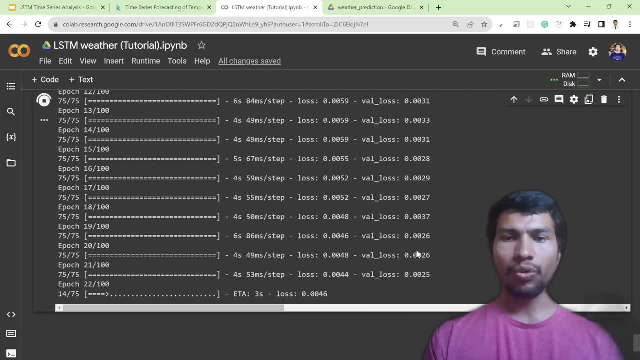 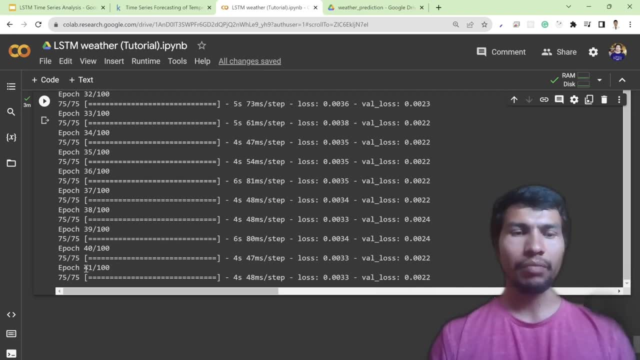 model and then it will only save the best weight. all right, so, as you can see here. so I initially set up my epochs number of epochs 200, but it stopped training at 41 epochs. so the thing is like it already achieved in the file loss of 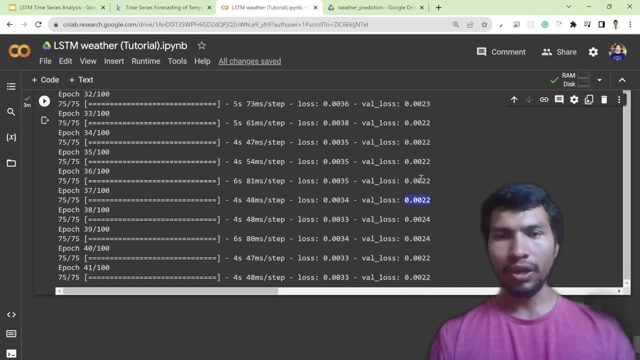 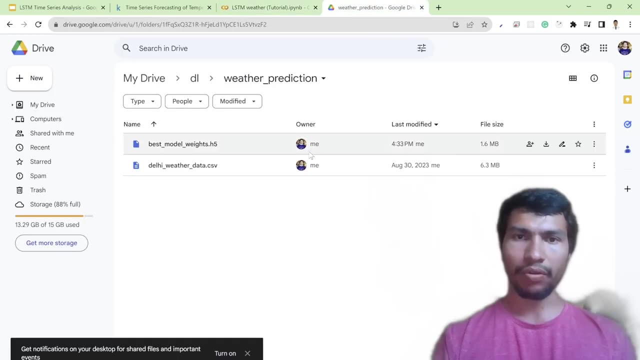 condition 0.022, and but after that it seems it's not increasing, it's up since it's not decreasing. that's why it stopped. like training, the model, so that's. and then of course our model is like model weight based. model weight are saved over here. 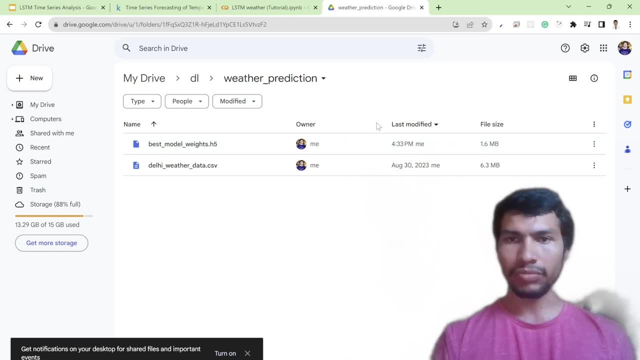 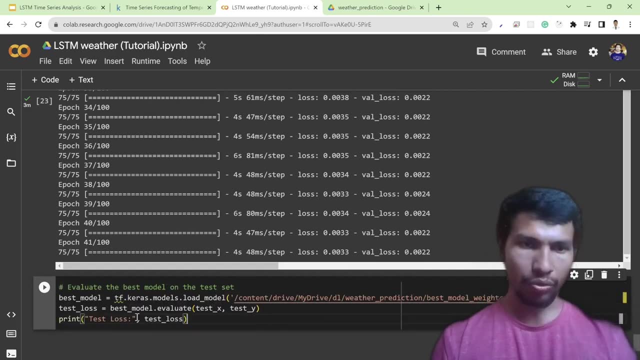 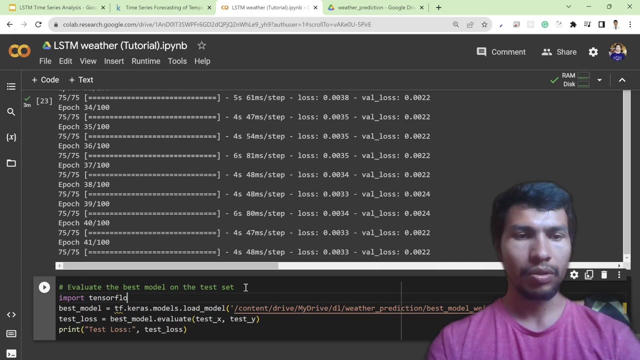 in the drive you can see the time. it's the current time and okay. so now it's time to like evaluate the model. so now it's time to like evaluate the model. so, okay, maybe I need to import tensorflow edge TF and then I'm going to load my 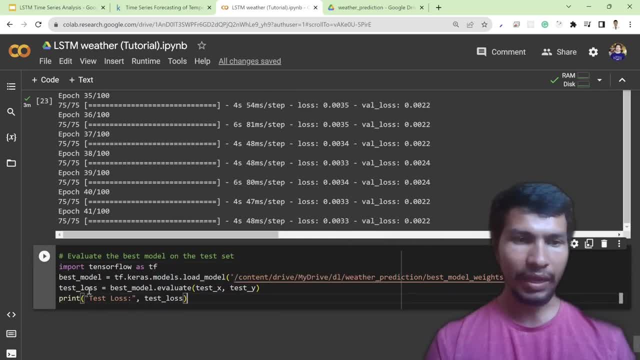 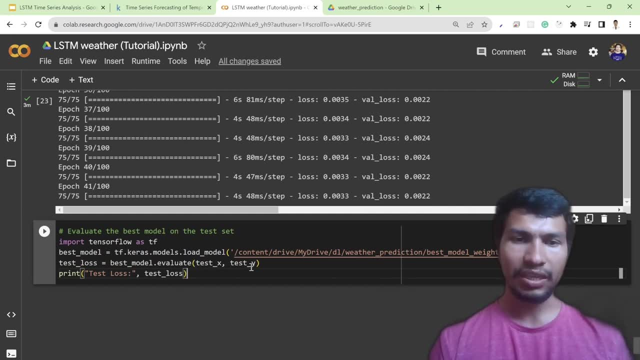 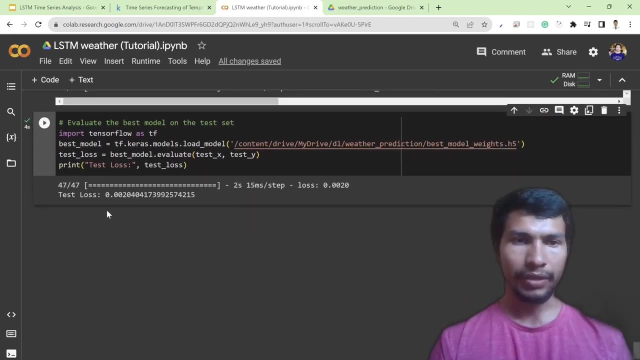 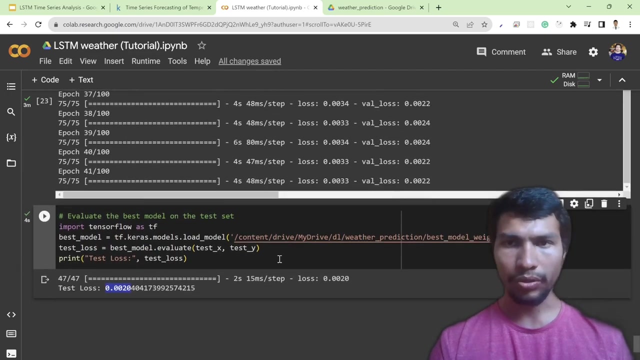 model from this particular directory and after that I'm just testing the test loss and based model dot evaluate test X and test y, and then test loss will be like printed over here: okay, so now I've like best weight test loss is 0.0020. so yeah, so now another thing I would like: 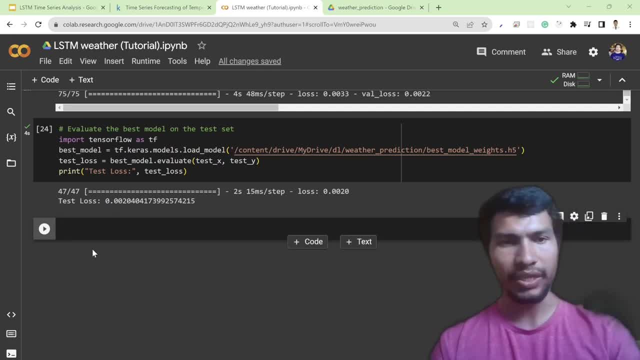 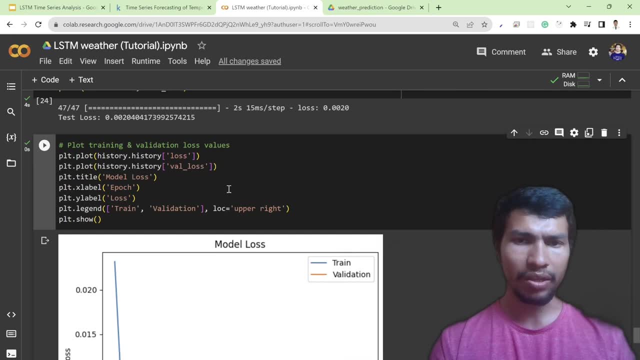 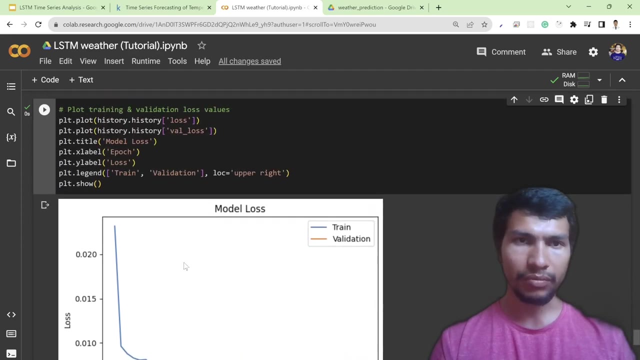 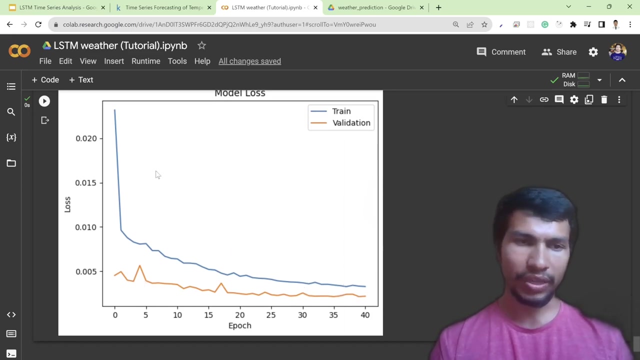 to like show you is the like history that means how our model is trained. so history dot history loss and val loss. so val loss is val loss refer to validation data set and train loss refer to training data set. so that's how our model is like trained. so you can see our like gradual decrement in the loss. so 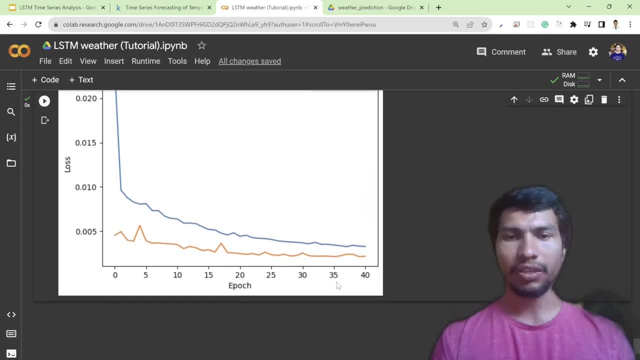 that means our model is training and then it's trying to like do the pretty good job, okay. so now in the thing is like: also, you can check other kind of like accuracy matrix. so in order to do that, you can check other kind of like accuracy matrix. so in order to do that, 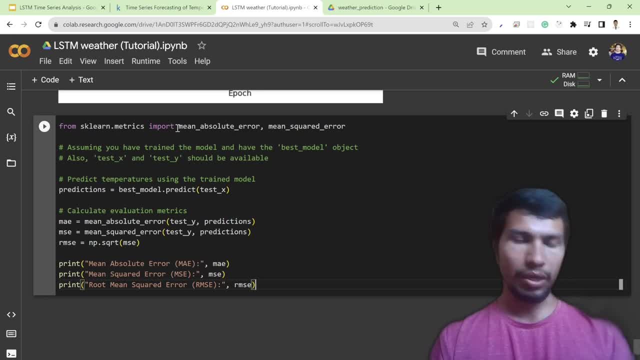 you can simply simply get some of the matrices from scikit-learn package. of course, here I'm simply trying to check the mean absolute error and then mean square error and root mean square error. so simply, if you run this function, so here I'm predicting the, my prediction based on test data set and then after 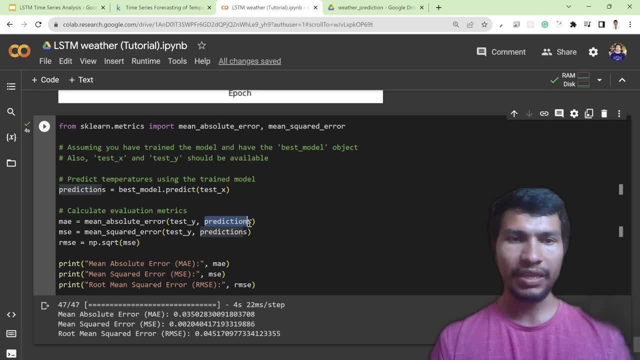 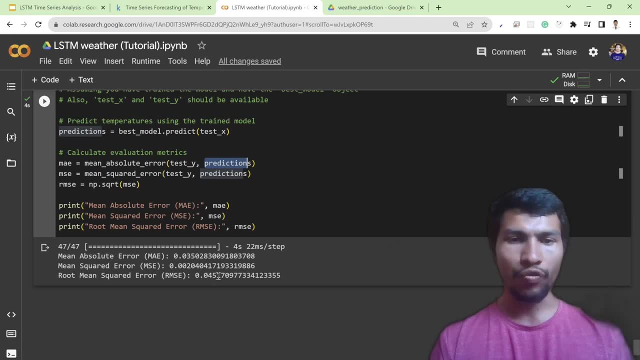 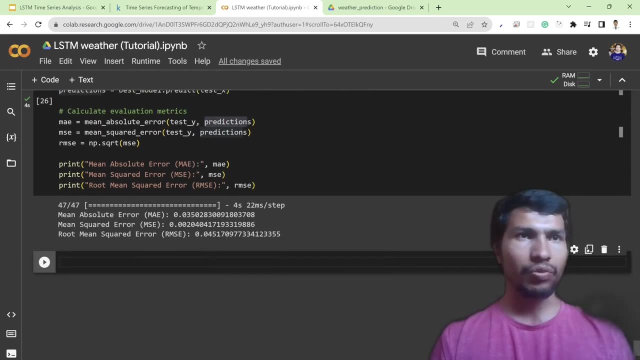 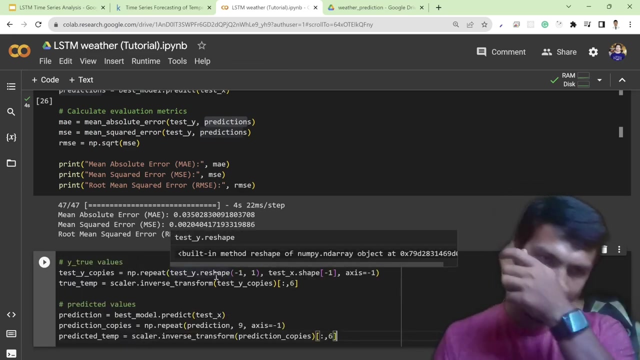 that I am passing my actual value versus prediction and based on that, we can get that like RMSE of 0.045, which is pretty good, yeah. so yeah, now it's like time to like predict and get the actual temperature. so, in order to like do the actual temperature, so we need- we also need to: 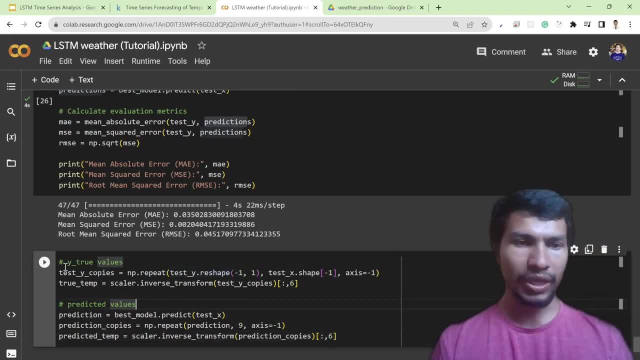 like reverse, inverse the transformation. so here what I am doing is like taste, why copies? so first of all, like I'm simply copying my test y values up to, like the, I think, nine times, ten times. because nine times? because there are nine variables at the beginning, and then I'm also trying to get the true temperature. 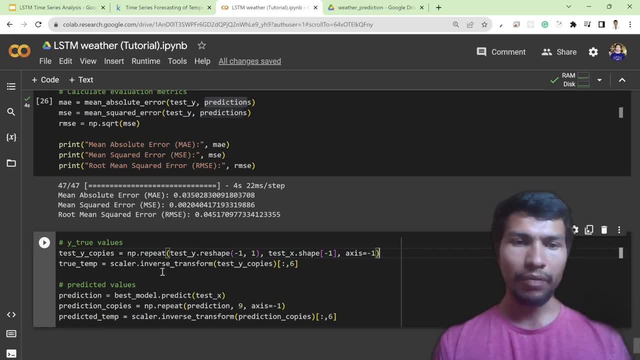 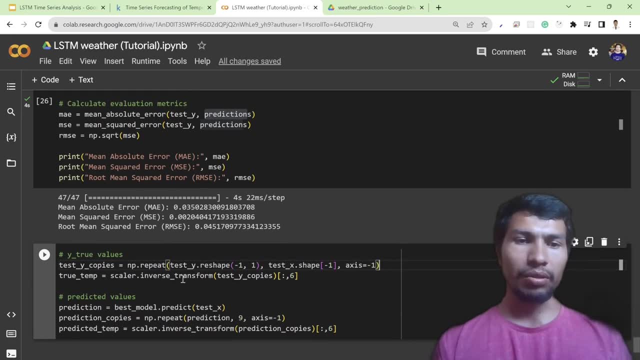 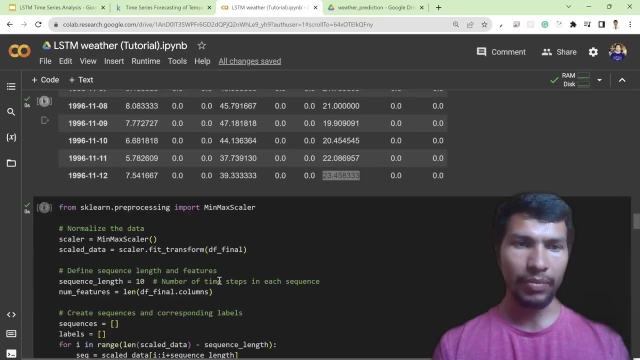 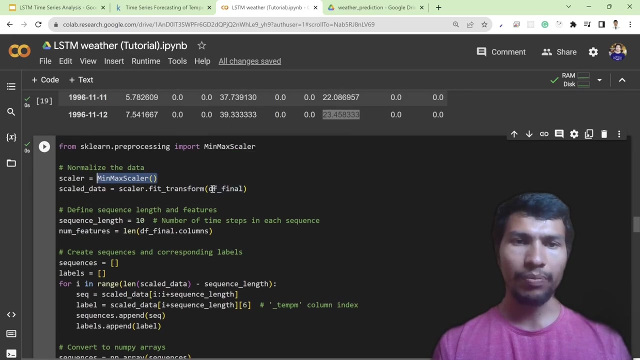 based on like scalar dot inverse transform. of course this inverse transform will like convert my actual like as you convert it to the actual temperature is I mentioned over here at the top. so we did some kind of min-max normalization right. so this our temperature will be: temperature value will lie between 0 to. 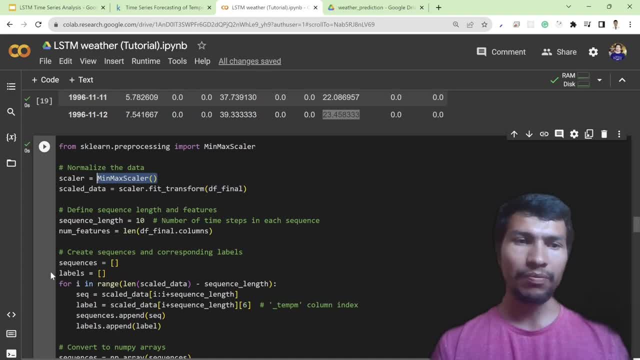 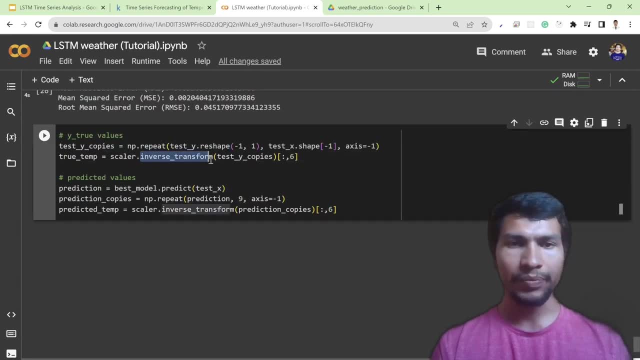 1. that's why we need to like, do the inverse transform in order to get the actual value. that's why we are doing you here, the inverse transformation. and then we are getting this sixth index, which is the temperature. and for the prediction, here we predict based on our test x. 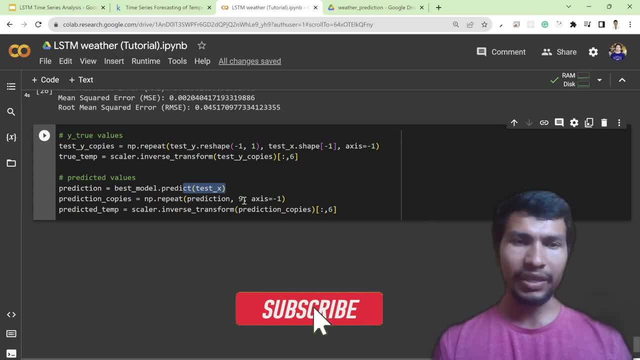 value, and then we are like repeating this nine times- that's the like number of variables in my model- and after that we did the inverse transformation and then we try to get the temperature. so yeah, so just hit, run and okay. so after that of course you can like, try to like. 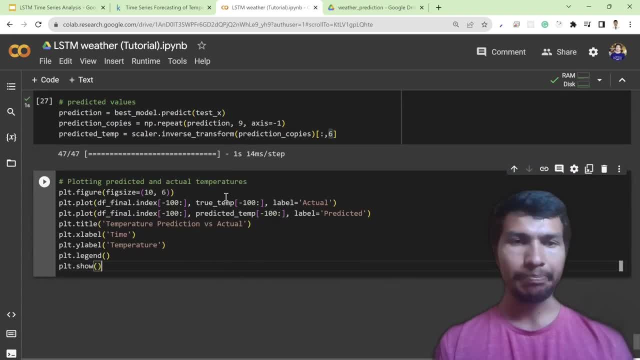 so then plot them in the matlock lip line chart. so here I'm just plotting the last hundred results. minus hundred means the last hundred index up to the last index, and then true value. these are like a, the indexes, that means our, like the actual date, and then this is my true. 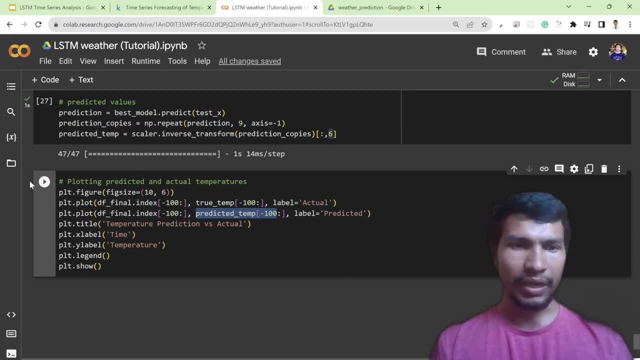 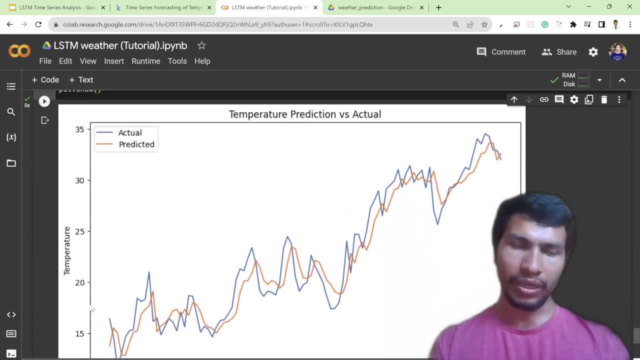 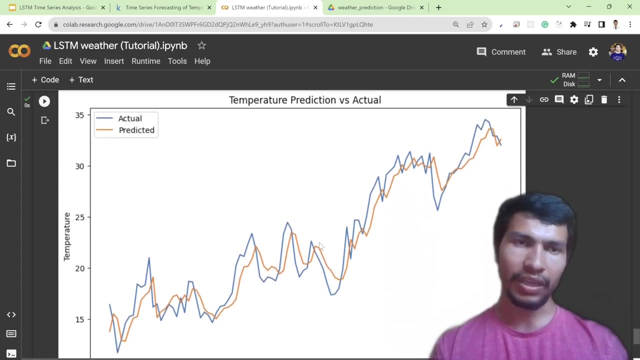 value and then this is my predicted value. and if I hit run so you can see this kind of graph, so it looks like, yeah, the trend is pretty similar, so it's it's doing the pretty good job in the temperature prediction. yeah, so, yeah, so, in this way, simple way,